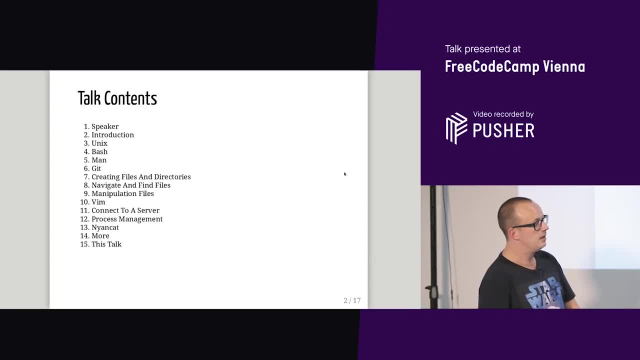 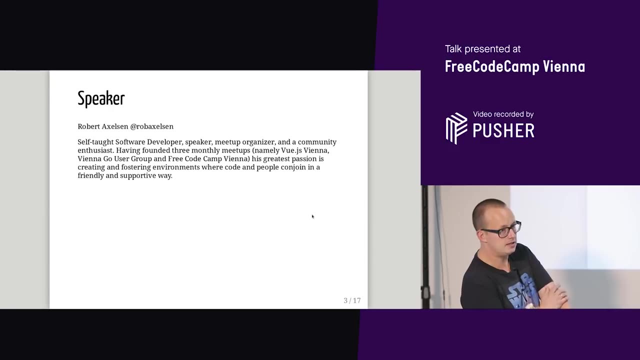 I will cover some things that I use on a bi-daily basis and we'll go into short detail of what the command line is and maybe why you should use it. I'll give you actually a little bit of info at the end about how I made these slides. 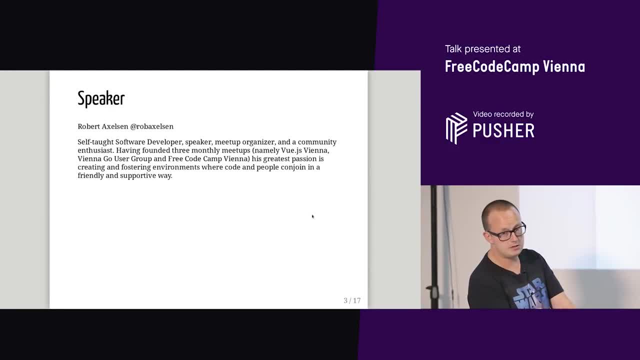 because that's also an interesting story. They look a bit different from the slides I had recently, so I'll get to that. But yeah, my name is Robert Axelsen. You can find me on most things as at Rob Axelsen. Coincidentally, I also have everywhere on all the things. 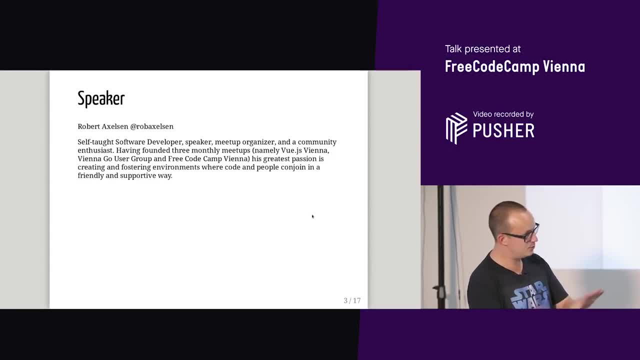 So I am at on all the things, at on all the things, But those are mainly aliases for now. Rob Axelsen is where I actually am. I'm a self-taught developer, like we talked about earlier. I'm a speaker. I'm a meetup organizer. 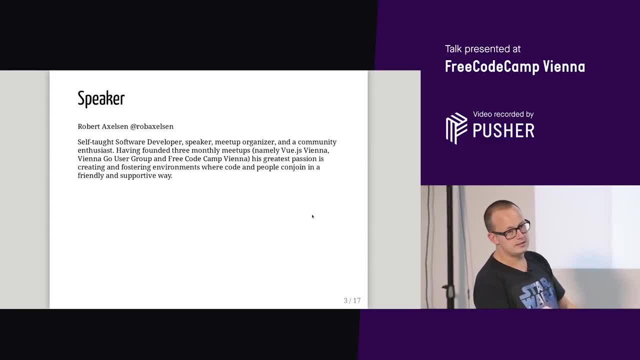 I'm a community enthusiast, And then there's a long sentence there, but all I want to say is that I love it when, just like today, when code and people come together, and I love to get to know people, help people learn to code. 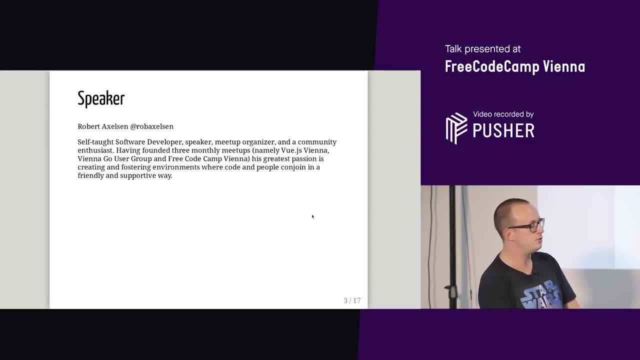 and be amongst other geeks and code enthusiasts- Awesome. So, as I said earlier, this talk is by no means meant to be exhaustive and I hope that if you realize something at part of the talk, you're like: oh, that's cool right. And I hope that if you realize something at part of the talk, you're like: oh, that's cool right. And I hope that if you realize something at part of the talk, you're like, oh, that's cool right. 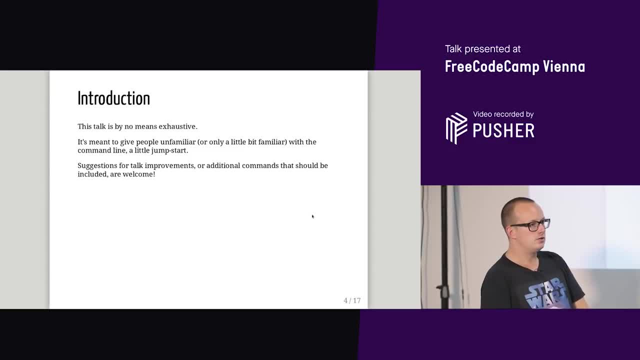 But he should mention this or that's wrong or whatever. Feel free to mention it to me afterwards or, even better, commit a pull request, because the talk slides are already online And this is meant to be mainly for beginners, people that haven't really opened a terminal. 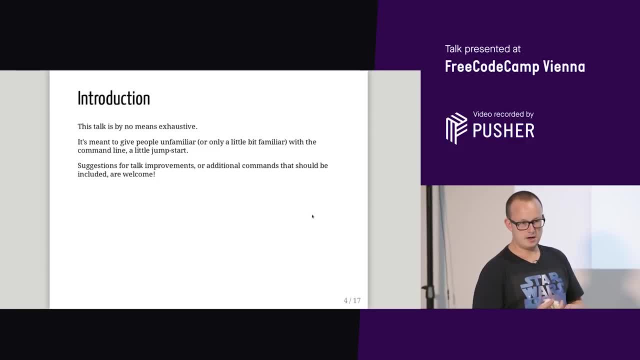 or the command line before, Or if you're a little bit familiar but you're not sure why you should use the command line more, or you're a bit too scared, or you're like, okay, now's the time to maybe get better at this. 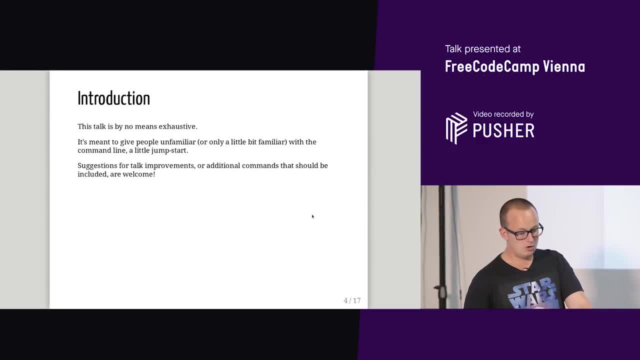 I'm gonna try and give you a jumpstart. Yeah, One thing that I think we should make clear first is in terms of the command line. The command line is just the opposite, or an alternative to the GUI, the graphical interface that you use. 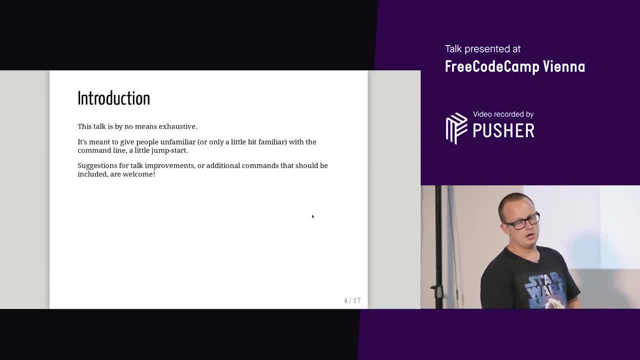 to do stuff on your computer. You might go to YouTube to watch videos. You can also download YouTube videos from the command line with commands. for example, You might like to use graphical tools when you are committing your source code, meaning you're creating some code. 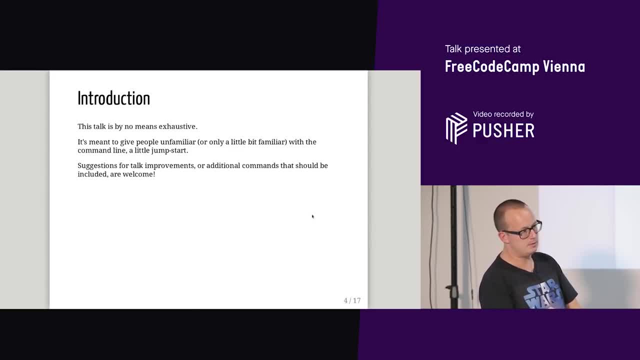 or you're programming something and you have a visual tool that helps you keep track of all of that. You can do that from the command line. You can play games from the command line. You can do all sorts of things, But for me it's mainly a way of being more aware. 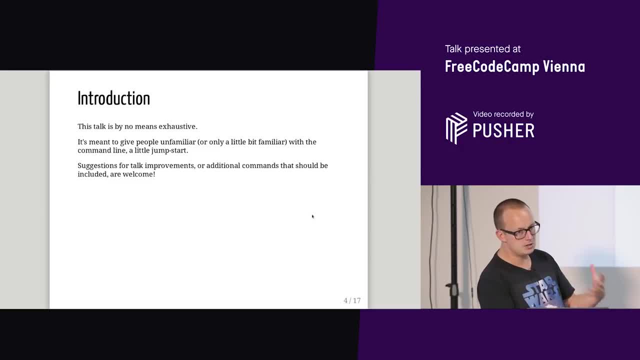 being more productive And as it becomes muscle memory, it also feels like I'm. it looks to others like I'm having magical powers, and it kind of feels like that sometimes as well, Because if you make the effort and it becomes part of your routine, 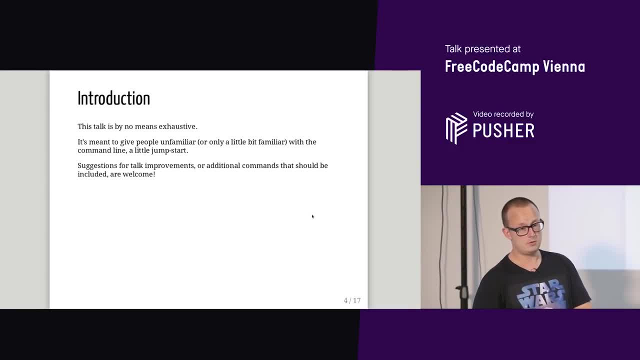 there is an initial steep learning curve, for sure, depending on what you're using the command line for. But if you're willing to give that an effort, you will benefit from it. And also some of this is stuff that you will. 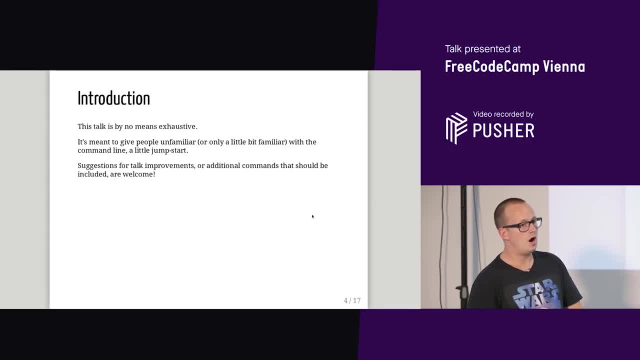 eventually have to know as a developer. Normally, if you are using an IDE or you're in a company where you have IntelliJ or some IDE which does almost everything and you just have some terminal inside the IDE, okay, maybe you won't really have to know so much. 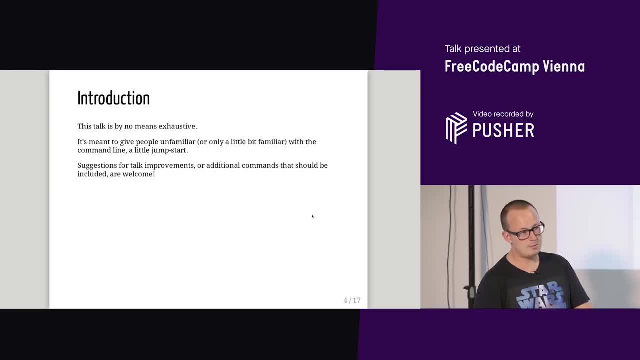 But at some point it will only benefit any developer or programmer to know some stuff about the command line, And some of the stuff we're sharing today will just be basic stuff. that will help you a bit if you don't know it from before. 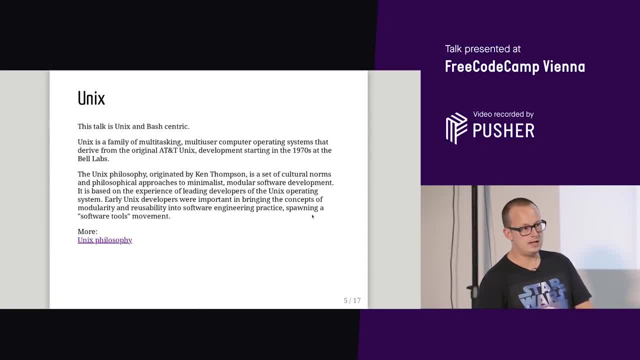 Command line can mean many things, and there is a command line in Windows. I won't go into that- unless you install what's it called Bash for Windows or something like this, where you get basically a Linux interface in Windows. 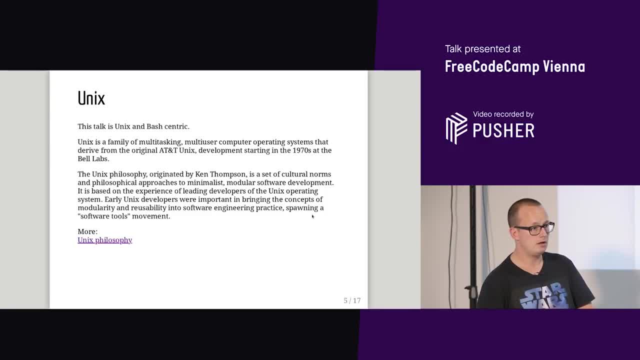 You will Sorry, SIGWIN is the name, SIGWIN. okay, Cool, cool, And you will also benefit from this talk. with some not disclaimers. with some exceptions, Most of this stuff will work on Mac as well. 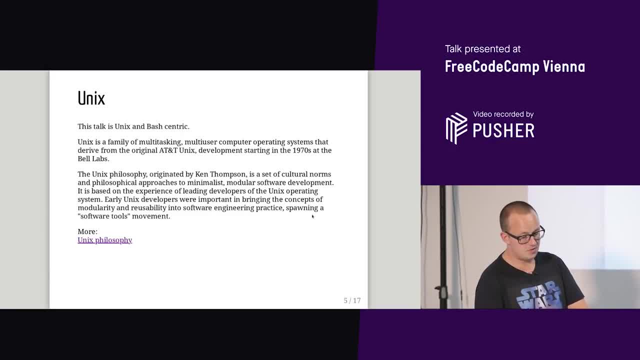 because Mac is also Unix-based, BSD-based. I just included some stuff mainly from Wikipedia here in terms of what Unix is, But it is in essence, an operating system that there are current operating systems that are derived from. It's a simplification, but that's all you need to know. 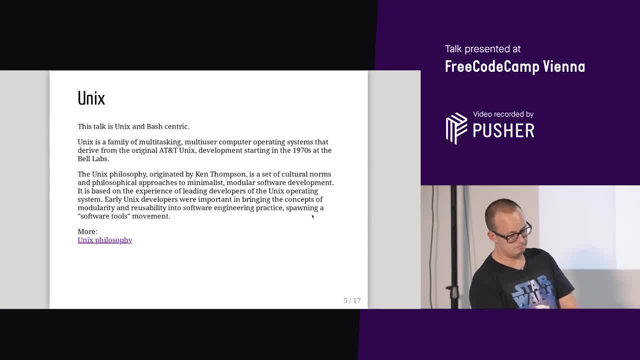 And one thing to mention, which we won't go into depth on today, but which you might notice later on, is that Unix has a philosophy of having modules for everything, and every program or tool should be really good at what it does, And then it can be chained or combined. 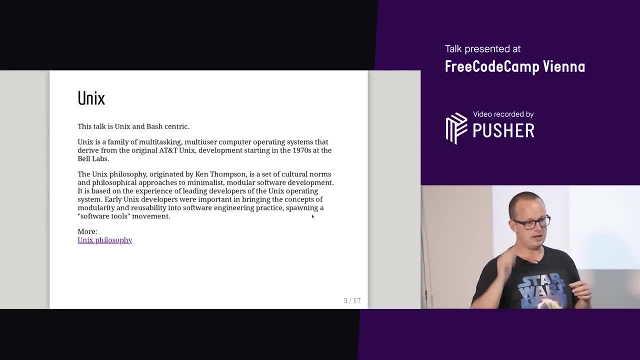 with other commands or tools and they together will do the job really brilliantly for you. I won't go into any advanced examples, but if you're interested in that kind of way of, yeah, Controlling your computer from the color and line, 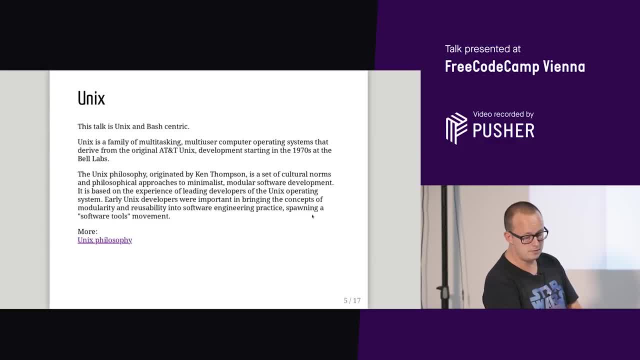 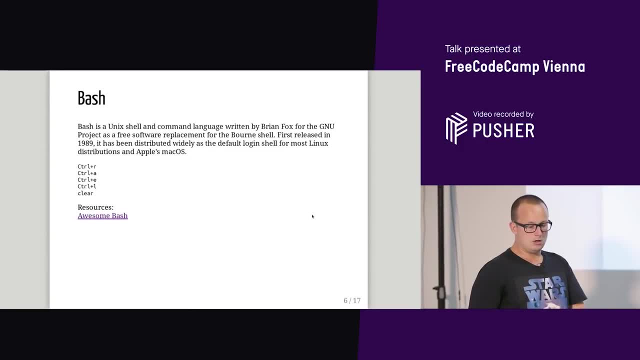 and benefiting from that kind of philosophy. that's a whole different talk topic, But it's just nice to know Not so much about Bash other than that we will. at the end I'll go through a little bit of demo. Feel free to save questions till the end. 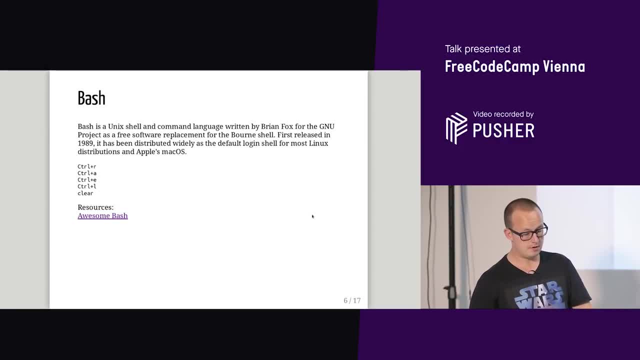 because of the talk it's not so easy to. with the recording, it's not so easy to have questions live, So please keep them in mind. Bash is a shell and command language, meaning the command line that you get up on Linux. 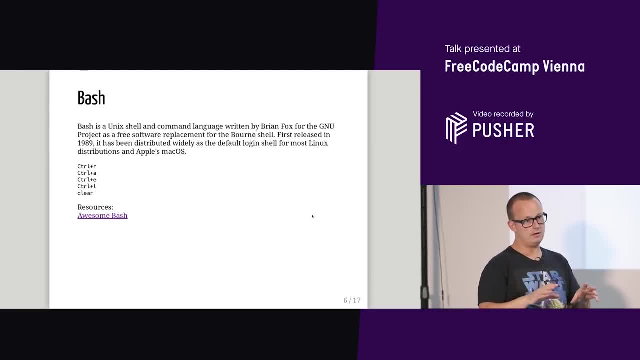 or Mac will be Bash-based And the commands you give outside of using a tool or a certain command with some options, those will be Bash commands. It's called born-again-shell and it's some. yeah, Enough said. There's a great resource if you wanna go into. 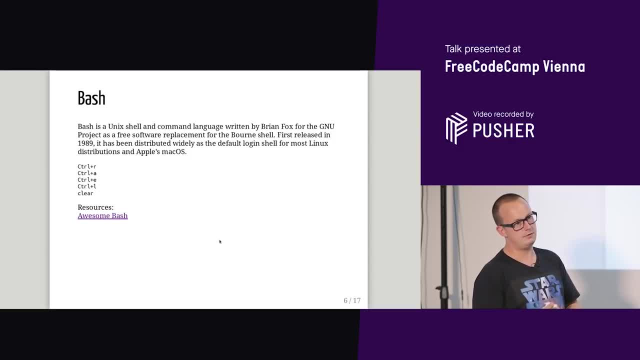 how to customize your Bash and make your command line look different, or program in Bash or whatever. There's a great GitHub resource which is called Awesome Bash, Where there's tons of resources, These commands that I've listed here: Control-R, Control-A, Control-E, Control-L and Clear. 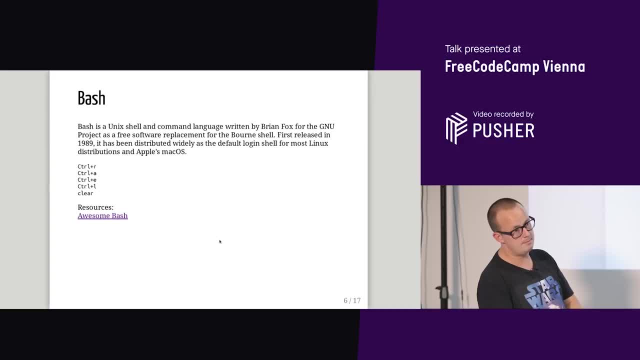 those are the ones that will make you the most productive in terms of using Bash. Those are Bash-centric Meaning. Control-R takes up all the previous. it has the history, your Bash history, all the commands you previously have done in the command line, I think. 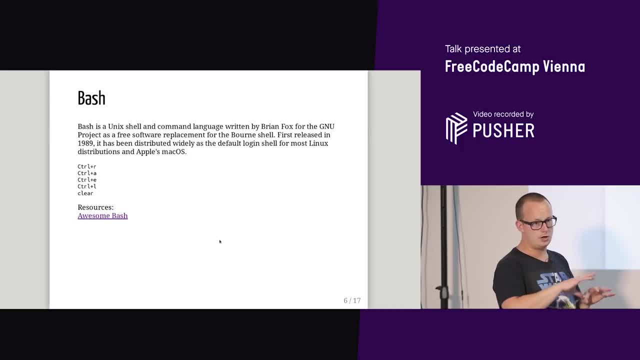 by default of the thousand last commands. Then you can basically search in them As you start Control-R, you can basically search in them. Then you can basically search in them As you start Control-R. you can basically search in them As you start Control-R, you can basically search in them. 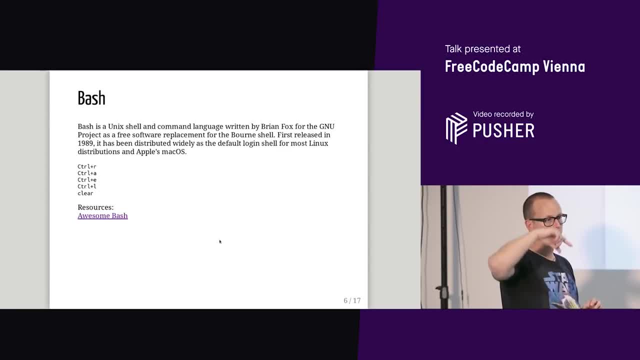 And start typing out. It'll give you the last command and then the history of the previous commands you've done. that started with the same thing: Control-A makes you jump to the front of the line you're on, and Control-E to the end. 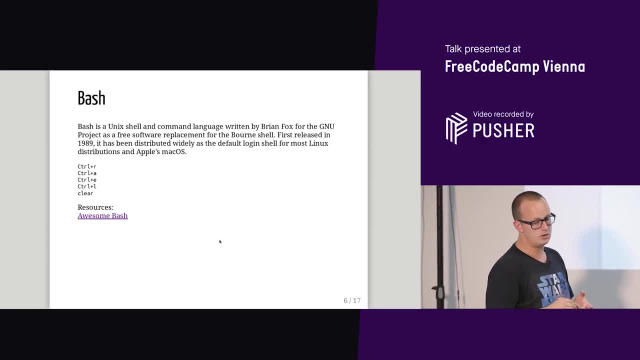 Feel free to code along or do this, but the slides are also online so you don't have to write down something. Control-L is the same as Clear. It clears the screen. You can also write Clear. Just write Clear, Enter, and it does the same job. 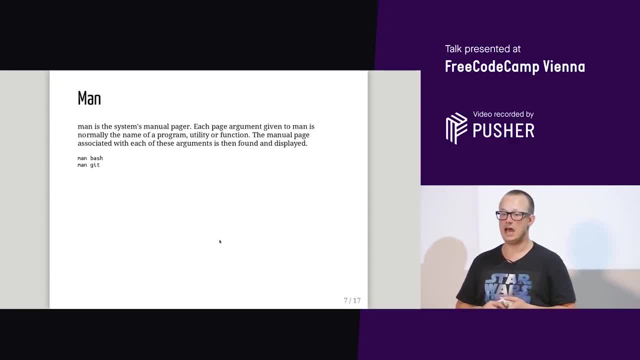 Before we start, Before we start, Before we start, just know that a good habit to get from the start is the man pages, meaning most every, for example, Linux tool, command line tool will have a manual page man page. 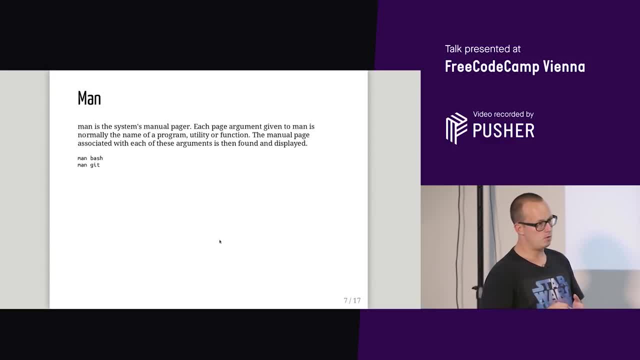 And you can normally just do man and space and the programmer tool that you are wanting to get more information on. So we're talking about bash. You can even do man bash and you'll get tons of information. Starts with a title, description, example. 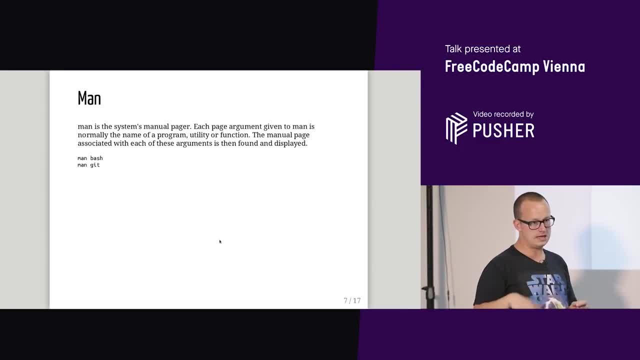 or the syntax, and it gives you the options and maybe some examples for those options. Options we'll get a little bit into later, but that's not really stuff you have to get so familiar with. just to get familiar with the command line. 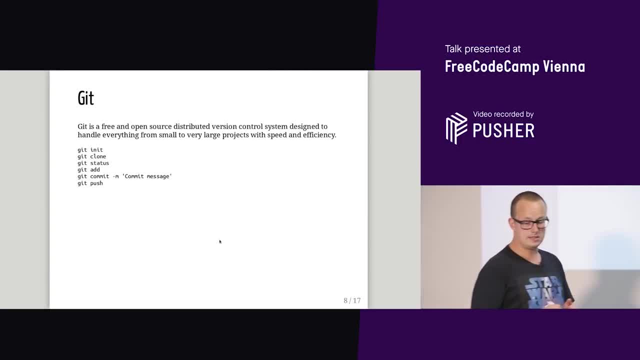 Git, as we talked about earlier with GitHub. that's a version control system and the most popular one to date by far. This is where you keep track of all the versions of the programs you write. If you code something, you might do something today. 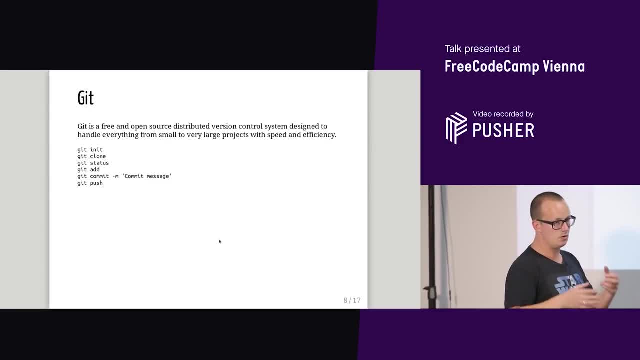 You commit it, meaning you save it. You save it locally, but you can also choose to save it, for example, at GitHub or a private repository, so it's only available for you. But you know that if your computer crashes, it's still there and you can pull it down. 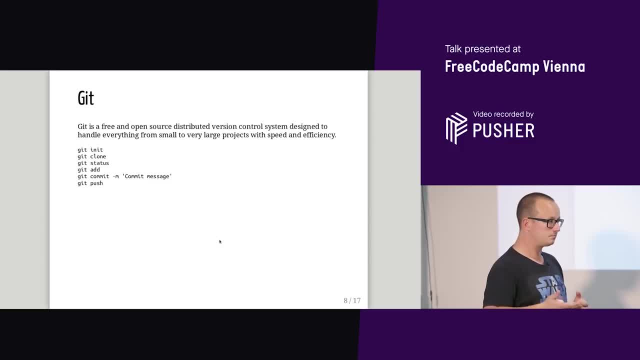 This also makes it easier to collaborate with other people, so that you can push your code. they can take that code down to make changes and simplify it. but that's parts of what this tool does, And all this you can do from the command line. 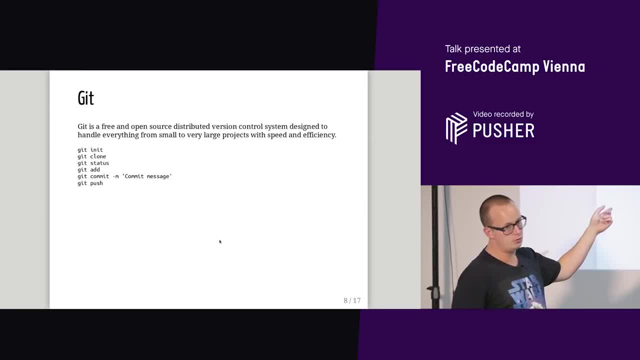 Sometimes you start with git init. There's a lot of code here. We'll go through those commands here. We'll go through some of the things together later And I know a lot of this is just throwing stuff at you and it might be wow. 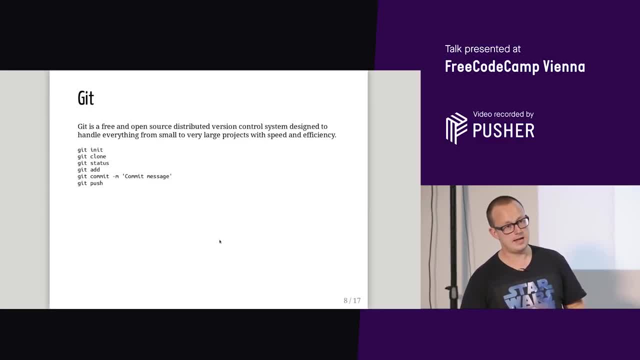 But my goal partly is if you remember 10% of these things and then you're in a situation where you're like, ah, I think I can do. that's hopefully helpful. Git init- you're starting a new project, Often if you're starting to learn to code. 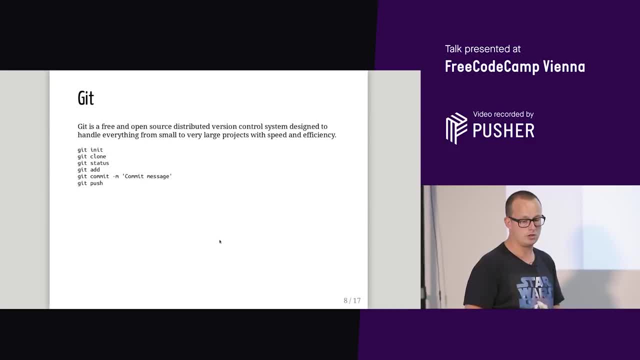 you do git clone instead, because you're putting down someone else's code, Then you normally get familiar with git status and git add. Git status shows you a really good overview and often gives you suggestions about exactly what you should do in that case. 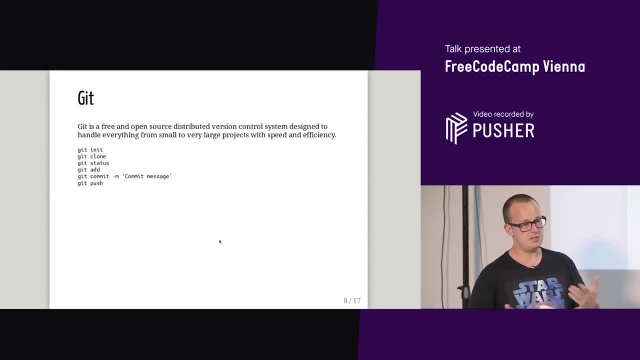 Git add lets you add new files or change files that have been changed. You add them to the stage, the environment. but let's not get into git specifics And git commit. that command means that you are storing the new version of your source code. 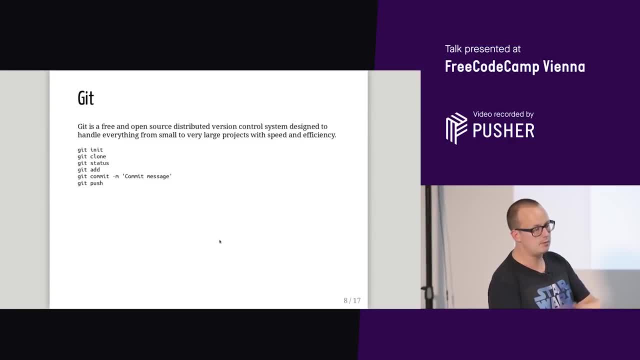 with a message that should be descriptive of what it does. And git push is when you're pushing it to locally or normally, a remote place where the code lives. But these are the codes that you like- 80% of your normal working day with git. 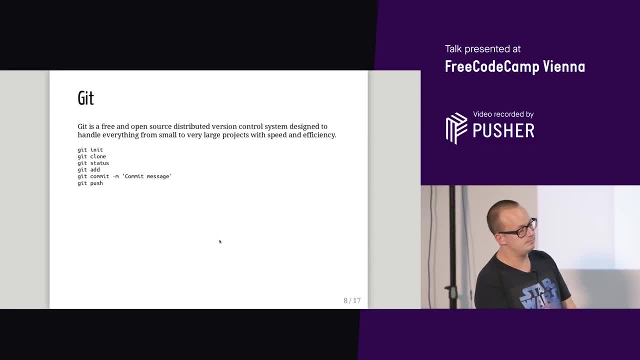 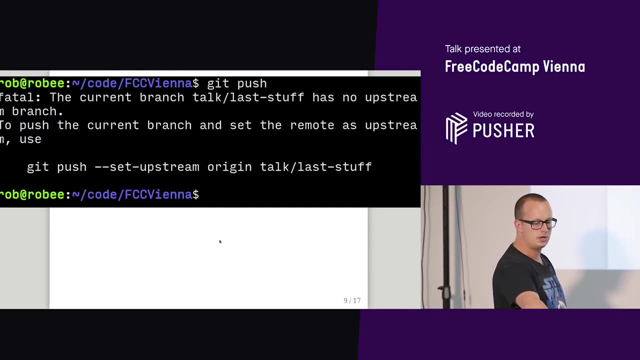 unless you have, like an advanced workflow in your company or with your open source project that gets you very far. Maybe to give some context, if I do this, I have a terminal window here that I use. that is a dropdown. We can show you how to open one, normally on Linux afterwards. 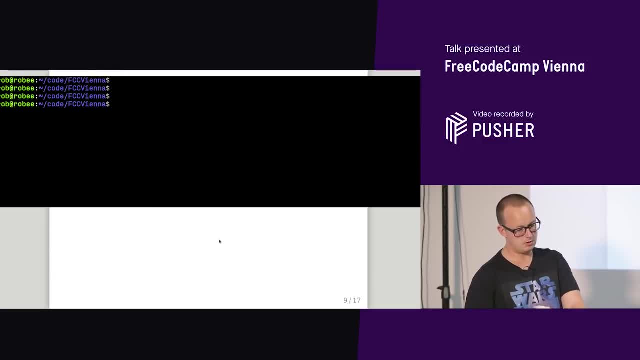 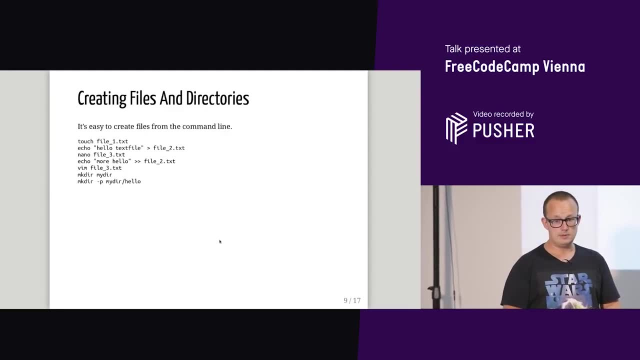 When I talk about the command line, this is what I'm talking about, just to give some visuals. if it was unclear, Then we can create files and directories from the command line. The easiest way is the touch command. Again, if you're curious. 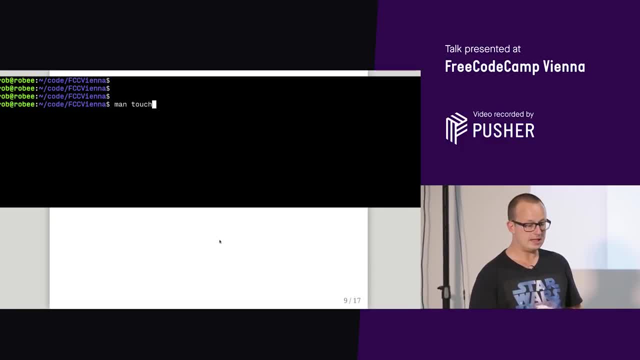 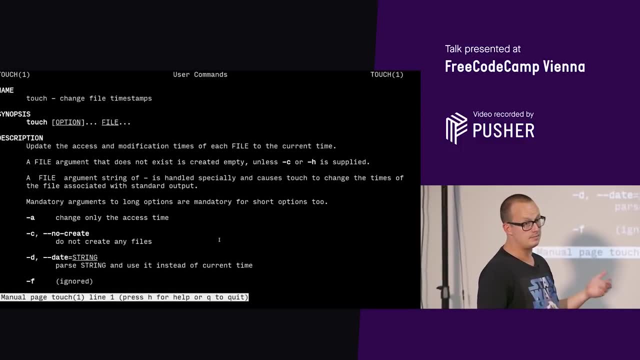 to give some more context, I can do man touch and it gives me information about what this command does for me, right? So it changes the file timestamps, but we can use it to create files. It has options as you see here. 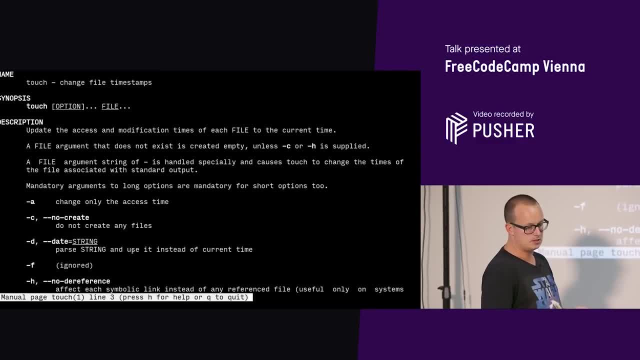 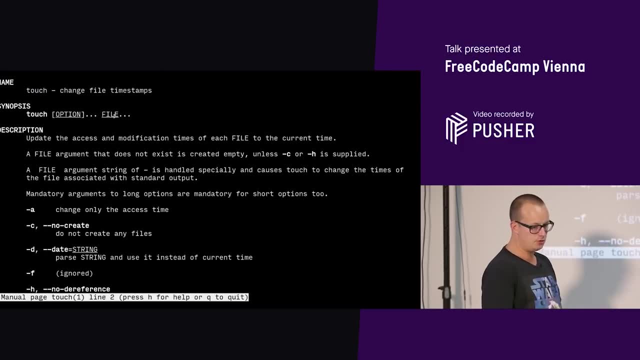 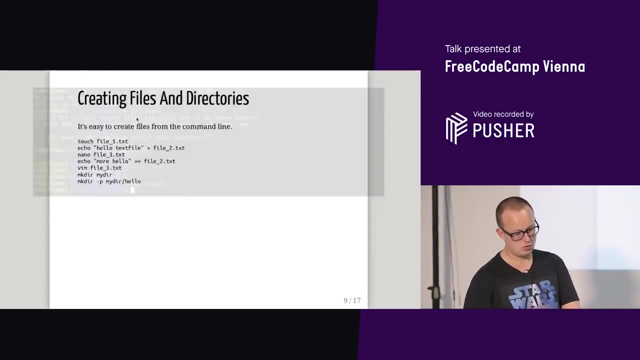 It has the description and it has the options and it gives us information about what they do And it says: you need to touch and you can do an option that's optional, but you need a file name. Yeah, So If we touch a file, 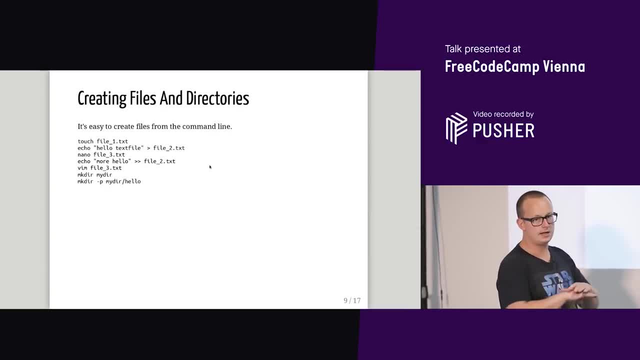 if that file doesn't exist before it creates the file. It's an empty file, There's like no bits, It's like it's just an empty file, And that's helpful sometimes. but sometimes you want to create a file because you already know what you want to put in it. 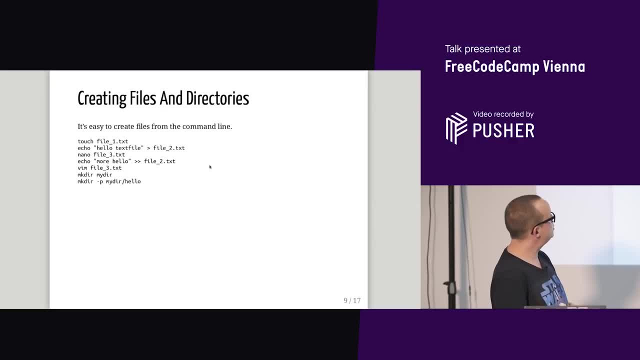 So from the command line you can use bash syntax of echoing out and then in strings whatever's going to be there and then you direct it to that file. That file will then have that content. There are text editing tools in your command line. 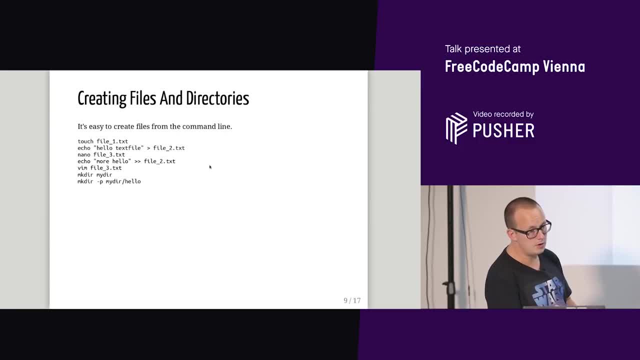 The simplest one, probably being nano, because you can follow instructions and stuff. We'll get to another one later, So you can also just do nano file tree and then you're opening a file and then you get instructions on how to save it after you've put some information into the file. 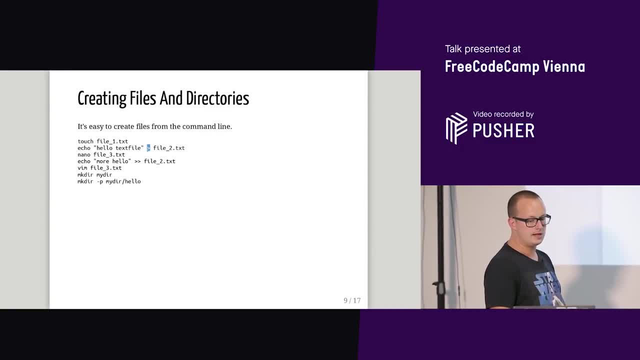 It's also important to know the differences, but I'll mention that this one overwrites everything in a file and this one lets you always append. So if there is something already existing in file two, this means that this will be added to it. 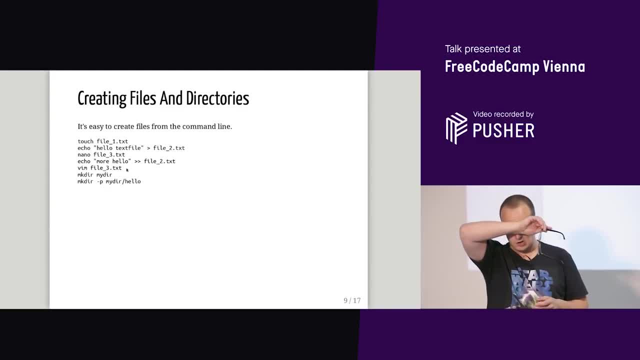 Vim. I won't go into detail today, but it's a more powerful editor than nano. Some people, myself included, use it to program all day long, So it can be a fully functional and more than enough productive IDE for you if you want to program. 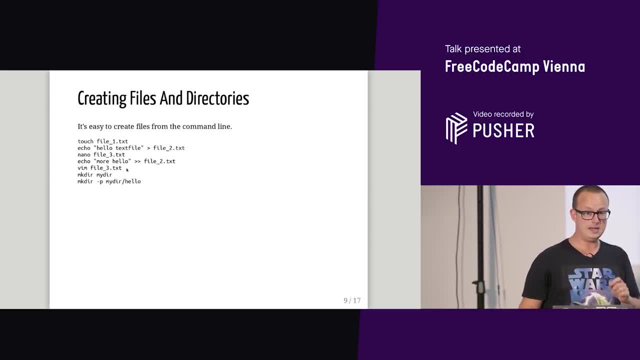 To make a directory you use: make dir, M-K-D-I-R. And one thing, one thing you'll use more often, if at anything more than that, is the P flag, the P option, which just lets you make more than one directory at once. 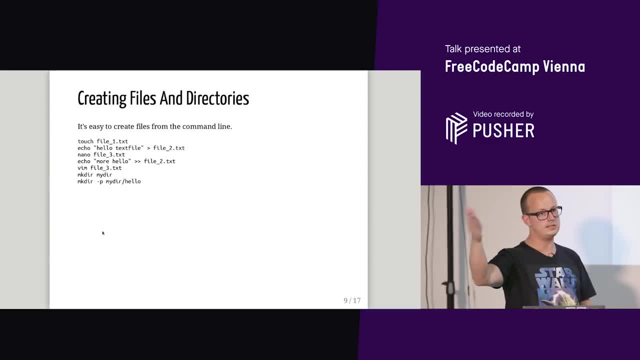 Because if you try without the flag, it'll say that directory you want to create a directory inside doesn't exist. Yeah, And now that we've created directories and files, we maybe want to have a look at them. So LS gives us a simple overview. 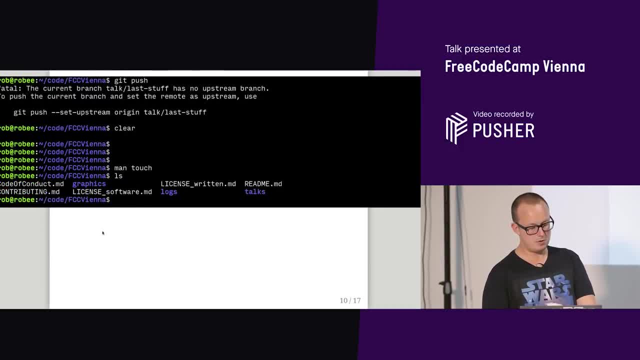 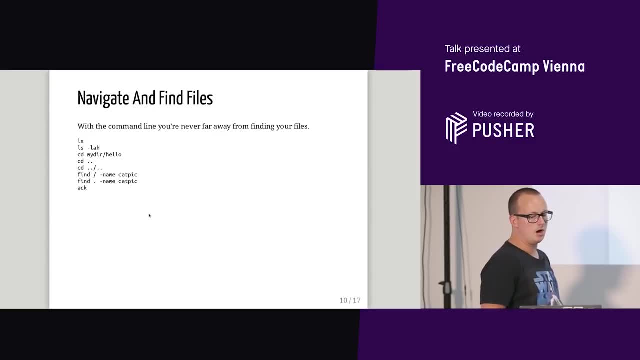 of where we are and what files are available, And LS again with options. So you see, here is an example of some tools. lets you have options or flags like L-A-H together. Some of them enforce you to have a dash in front of all of them. 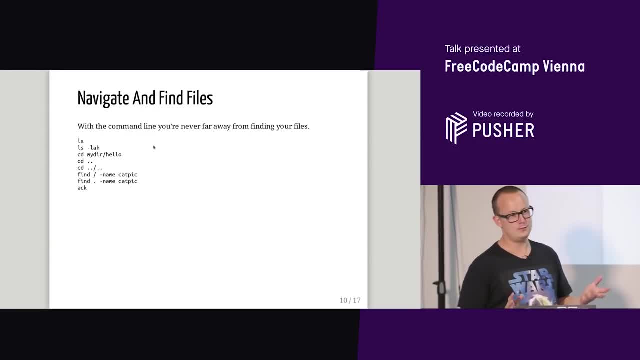 There is a bit of inconsistency between commands and tools, unfortunately, So it's good again to check the man pages If there's one thing you remember today from this talk: if you get confused in the command line there's something you're supposed to use just to man. 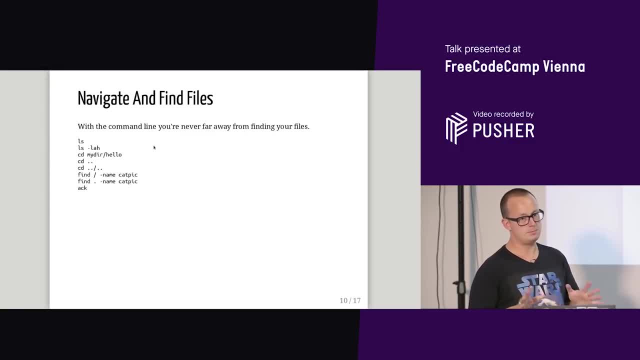 before the command and see what happens. You can get a lot on just by looking in the local information you have available for you. L-A-H is an example of list them not just in a row but as a list. list the files as a list. 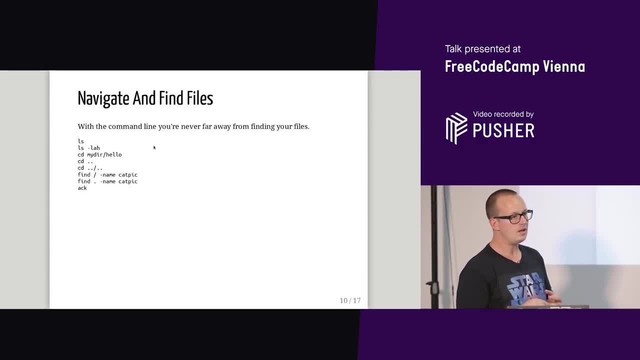 LS lists all the file in your current directory A. Thank you list all A for all. And H is human readable. So if you get all the sizes in bits and you're like how many megabits or whatever, is that? 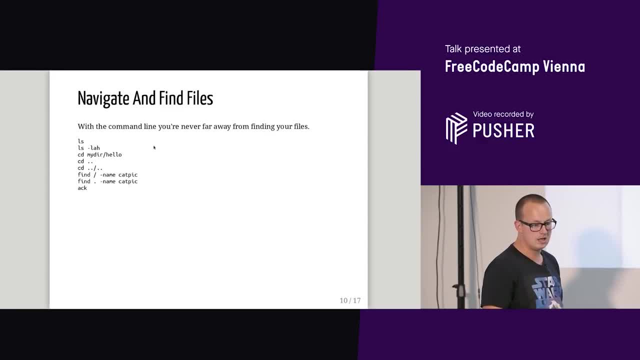 Then you can use that option: CD dot dot. when you are already, no, sorry, We go into this directory. so we have a directory, my dear, hello. we can do either CD my dear, then again CD hello, or we can do the forward slash. 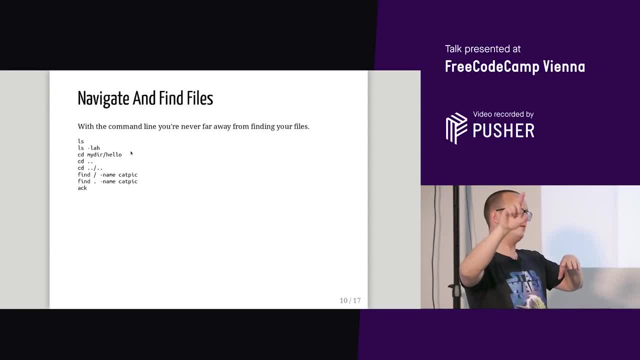 because it's my hello, is a directory in my dear. Once we're in there, we use the dot dot to go one directory back, And we can do a slash dot dot to go two directories back or two levels, And then we can do that infinite. 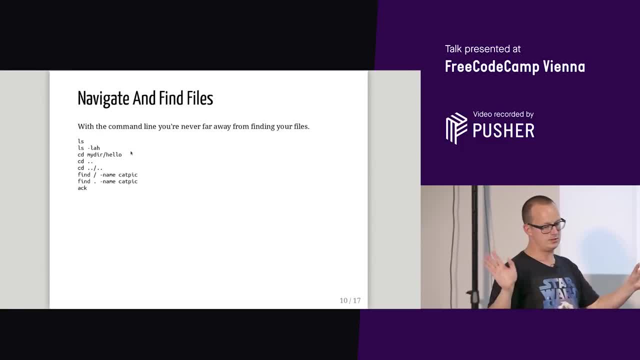 like as many times as we have like. there are some file system limitations, I think, but I don't think you'll run into them. I think it's more long file names. Find is the simplest command that is always there to find a file, so forward slash will find everything. 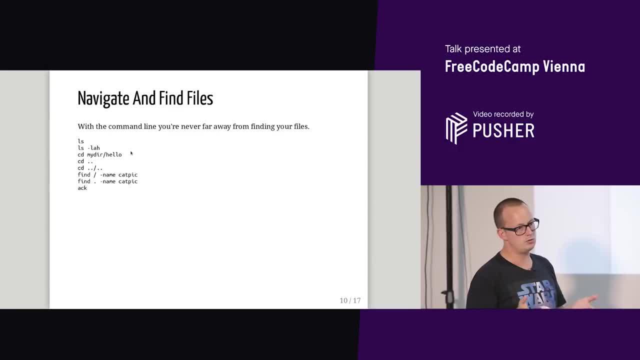 in your computer and the name denotes what you're looking for, as the name And the dot is from your current directory and downwards or up, yeah, downwards, upwards, whatever, I don't know, At least inside that directory and all the directories inside that directory. 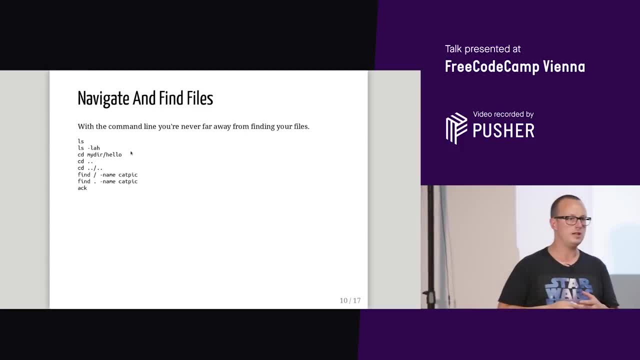 And one thing I maybe should put a resource here. but if you wanna install a tool that makes your life easier in terms of find, just install ACK or- and help me remember this- you can also do FCF, which is a Fuzzy Finder. 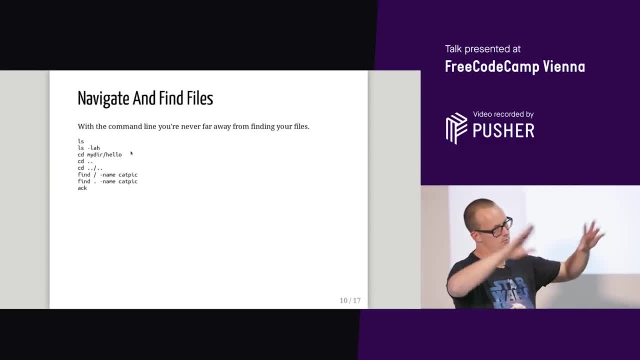 which you can replace the control R with this, and it's even more powerful in terms of finding not just your history, but it has also other combinations of stuff where you can find based on file name. To confuse you less, Fuzzy Finder just means: 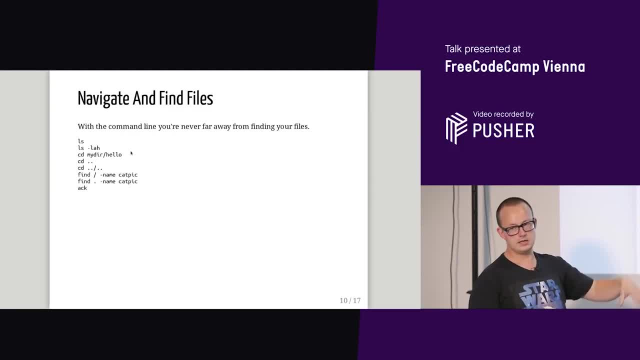 you don't even have to type out the full name. You can like. if something is cat pic, I can write ctpc, And because that file name contains those, I can do quicker, like a fuzzy search, Manipulating files. I will get to some examples afterwards. 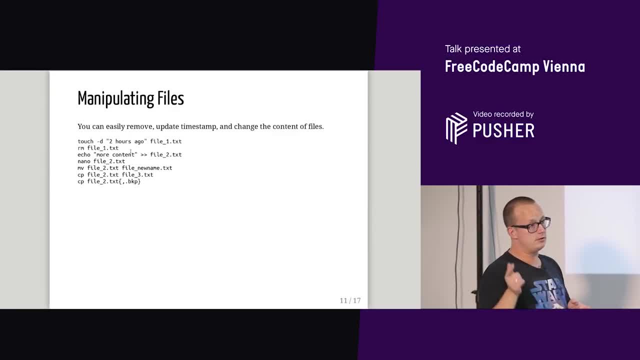 It's getting really tough now, but bear with me. Getting back to the touch command, if you do the option D, you can specify: actually now we don't wanna create a file, We wanna take an existing file and we wanna give it a new timestamp. 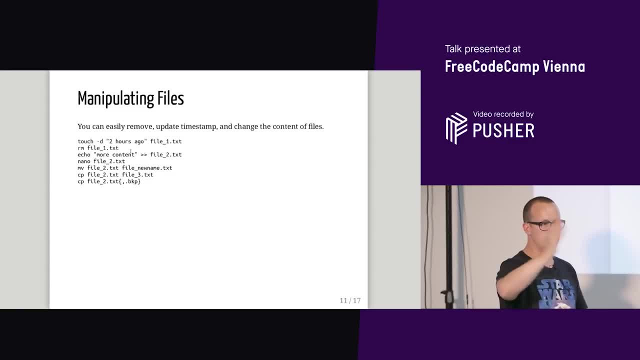 meaning we created it four weeks ago but for some odd reason we want to make it appear that we created it two hours ago. So then you can just specify a file and you can do touch with the flag D for a date stamp. 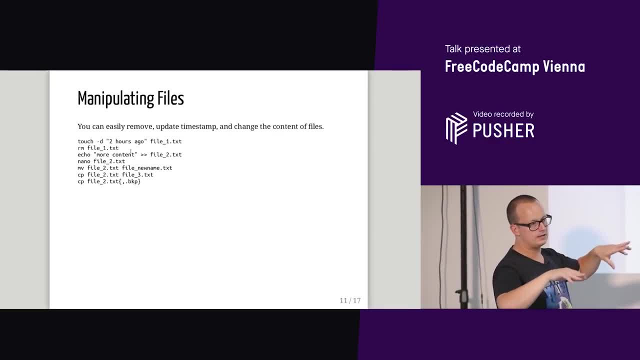 I think, and then you can even specify in like clear tags two hours ago, and you can also do date formats- and then the file you wanna change And then in like both on Linux or if you copy it to Windows. 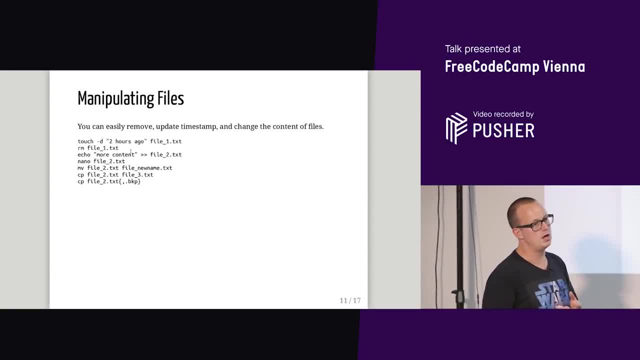 it'll appear as if it was created or no, as if that was the last time it was edited. modified Rm removes the file Rm. don't play too much with Rm if you don't know what to do. 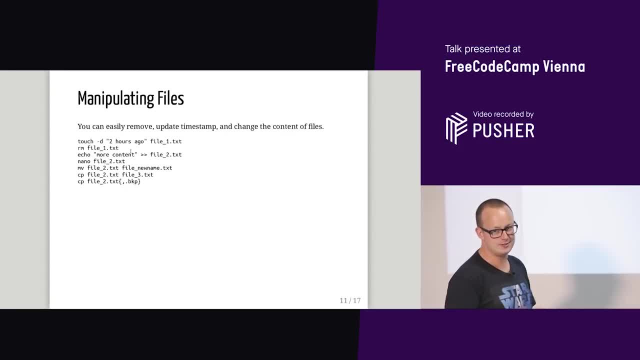 You can do stuff like Rm, Rf, which removes and forces and doesn't don't ask you for confirmation, And then you can do the forward slash, like we just looked at earlier, the whole computer, and then you have a. then you're gonna have a good time. 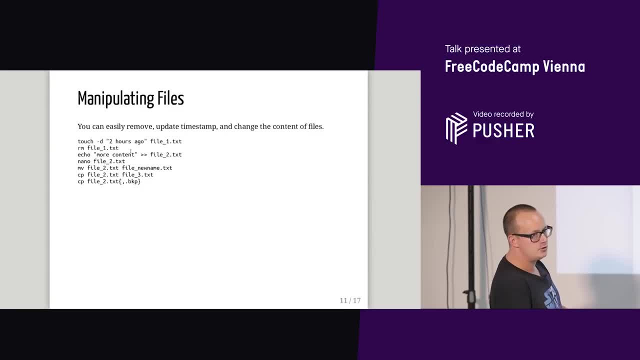 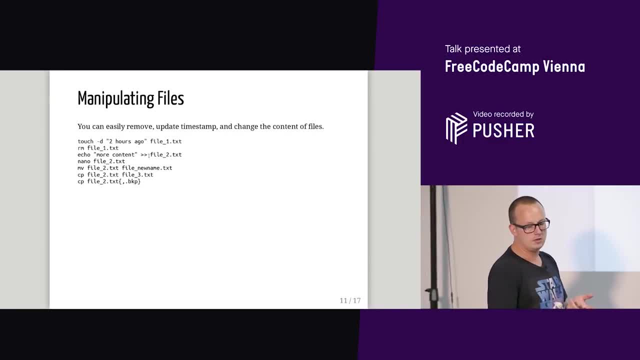 Manipulating files. We had that in the previous slide, but you can then with this redirect, you can only append, so you're updating this file to have a new line with more content. Again, non always useful if you wanna change files. 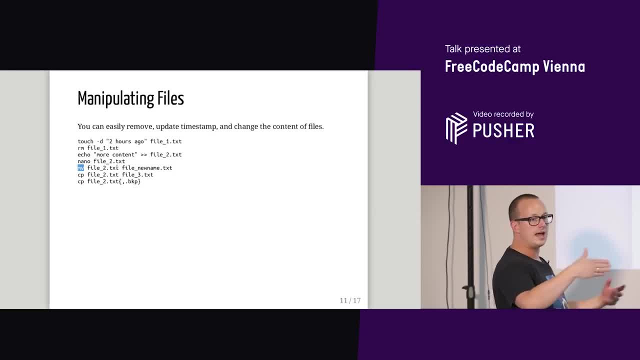 You can change the file name with just mv, which is its own again, you know Unix philosophy. mv does one job really good: It's good at moving files, changing names, doing that stuff really good. That's what it does. 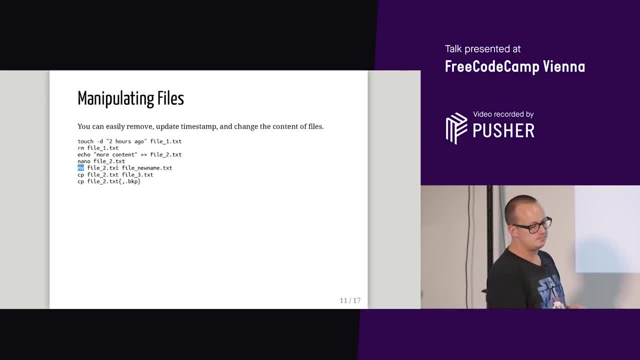 It's always there for you. Man mv. you get all the options. Man mv. you get all the options. Man mv. you get all the options. So you move it and then you can change the name, So the existing name and the new name. 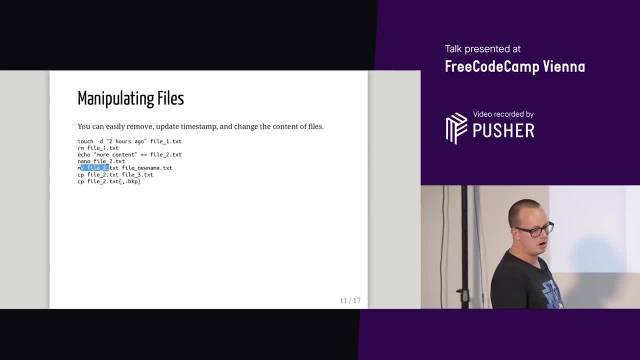 You can copy a file, so this would move it. File two would be gone and file new name would be there. Copy would then copy this one and copy it into file three and both of them then exist. And a nice trick if you do backups. 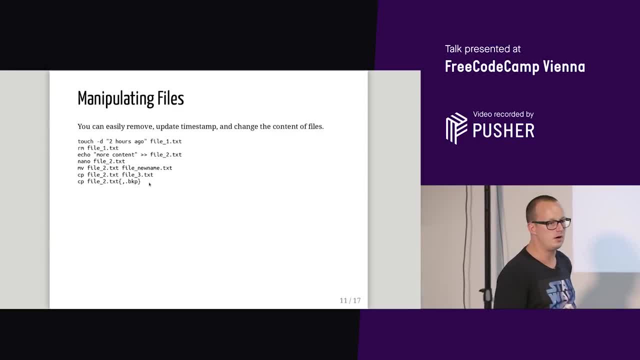 and you're often like: oh yeah, I just wanna backup this file and change it like config files or whatever you can do. copy file two and then you do some. don't quote me on this, but I think this might be Perl magic. 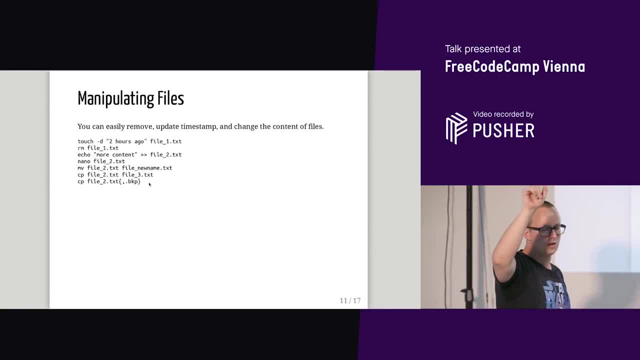 so it might not be fully bash, but you do the curly brackets, comma, dot. backup Means that it could take some parameters before the comma, but now we don't give it anything. so we're just saying: take the file name that you have and create a new file with that same file name. 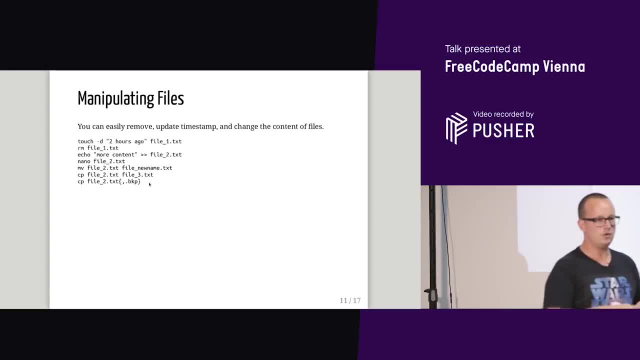 plus dot backup, dot bkp, for example. So if you use that and you get it in your fingers, you have a quicker way of copying a file if you always wanna do dot b-a-k or b-k-p or whatever for backing up that file. so you know if you make changes. 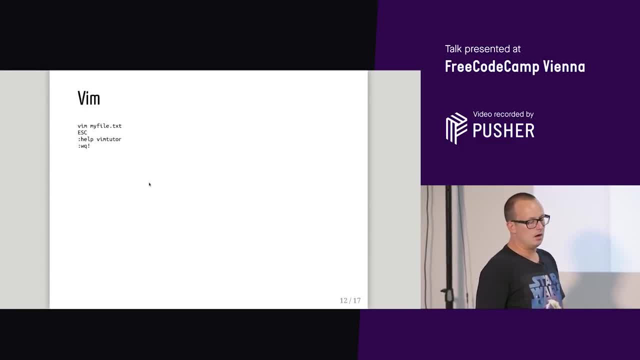 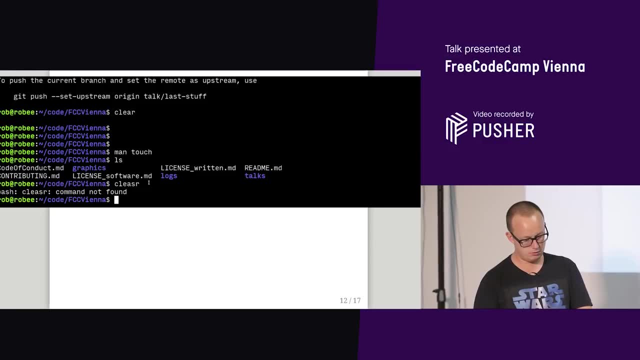 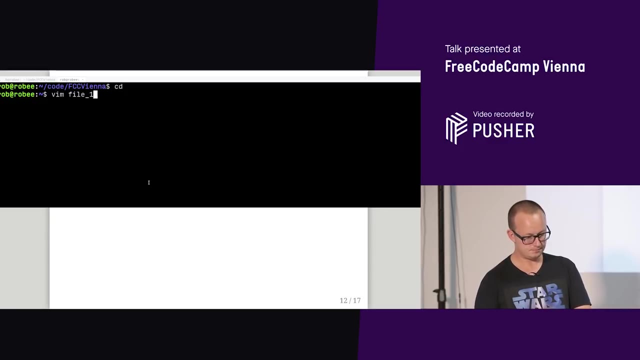 and you wanna revert, you can just yeah, Vim, I think I have to show some stuff here, because if I just do, if I just vim, file one, right, This is a text editor. Okay, what do I do now? 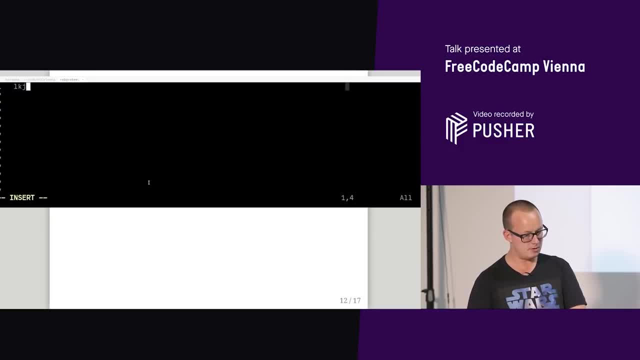 This is really not apparent, Like I'm just clicking random buttons now and suddenly something happened because I clicked the button i, which means insert mode. If I do escape, I can do a colon and I can do commands. here I can do help and stuff. 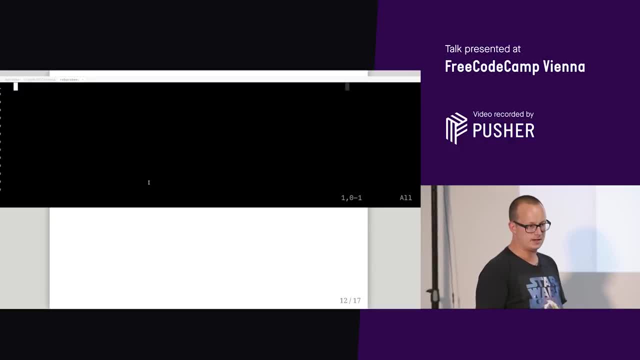 So it's not the most intuitive editor, but it's really feature rich. The best way to get familiar with it is just to go help vim tutor and then you get a file which leads you through: like, do this this way and try this out stuff, and do it on this file. 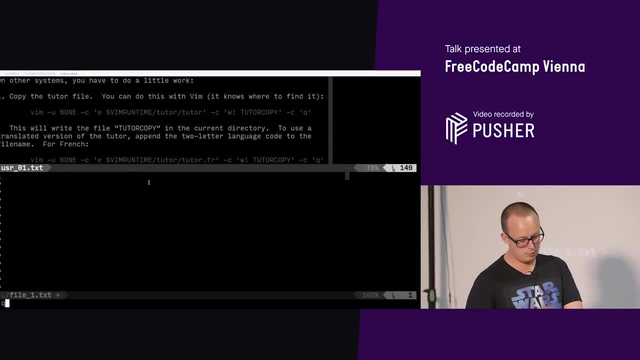 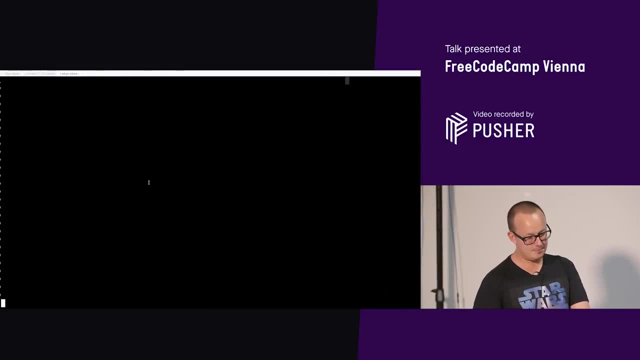 and you learn as you go along. But I don't wanna spend too much time on this, but maybe one thing to just remember really good is that I don't manage. so there you go, is that? if you wanna escape this, let me just blow this up. 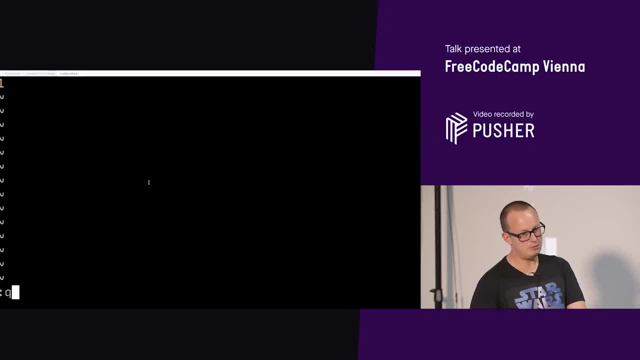 you literally just have to remember q and you might have to remember an exclamation mark, because if you don't, aha, Because sorry, because if you don't, then it'll tell you you did change. oh yeah, it will work if it was empty. 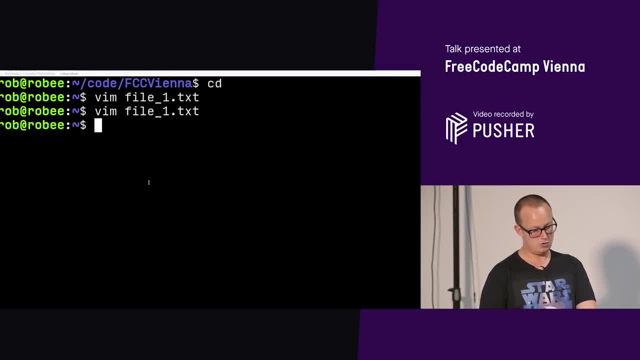 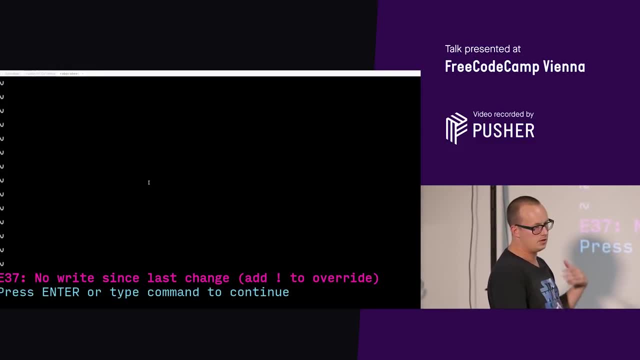 So it'll work now, Woo hoo. But if I did a change, it won't work because there was a. you changed something in the file since you last wrote to it, So then the safest way is to always know that it's colon q, enter, and then you're safe. 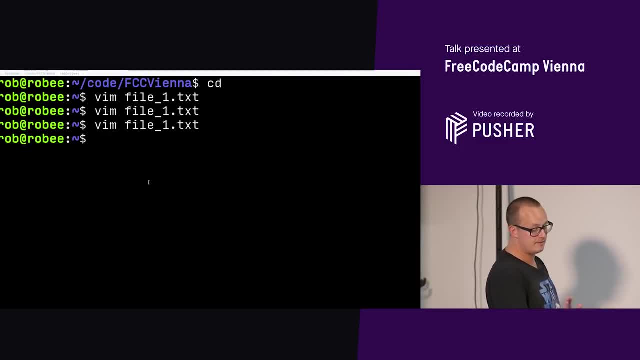 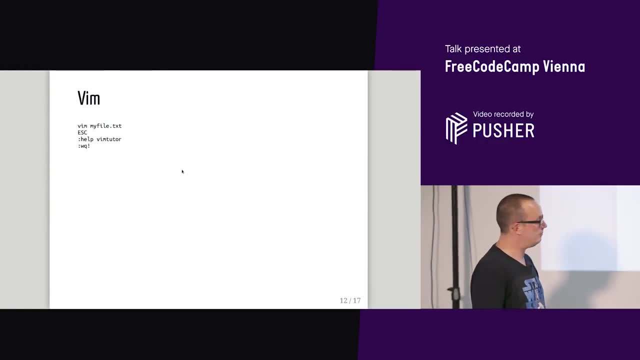 because then you can exit vim. You learned today how to exit vim and use man pages. I think that's more than enough as a takeaway. And the escape key is your friend. I've gone so far as I've switched permanently my escape and caps lock key. 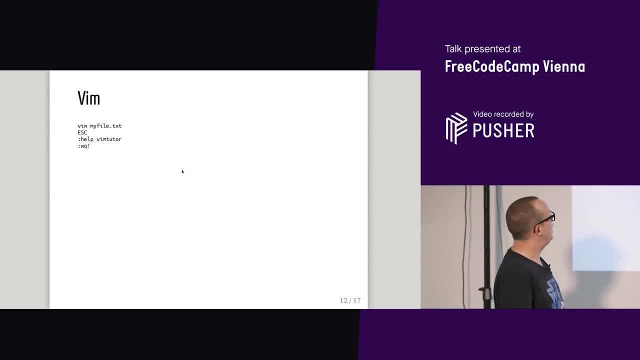 because caps lock is closer to my finger. Pardon, the French sucks when I use someone else's computer, but it works, Or someone else uses my computer, So we'll actually do some of this example. in the end I have to get up the IP address. 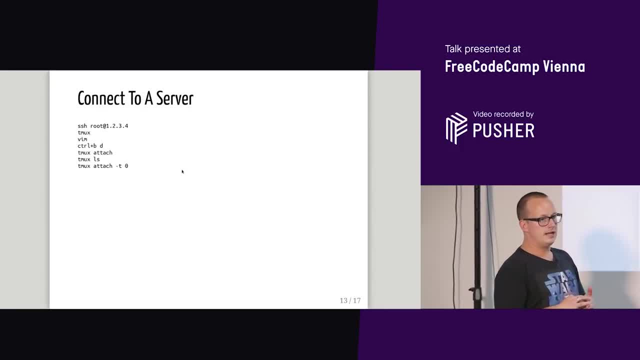 because I have a server ready for us. I just want to mention that for some of you, when you get into the back end or if you do some coding, you want to put your code somewhere, you might have to deal with another server. But the command line, the server, is maybe just. 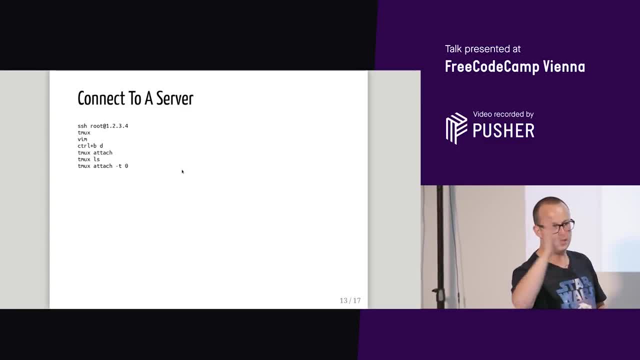 you interfacing with another computer and you do it most often, like 98% of the time, via the command line, Unless you're on Windows. for example, the stuff that you do on the server isn't often a lot of the stuff you would. 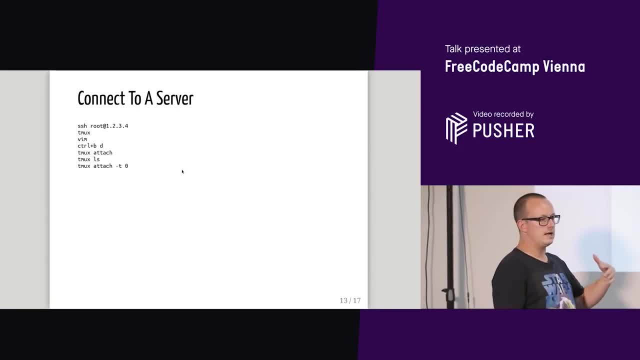 do on your normal computer if you use the command line. so this is an example of going SSH, meaning we're connecting a tunnel through a server secure connection where we can then use the command line locally, but through the SSH tunnel on the other computer. tmux is a great tool that enables us to, if we just 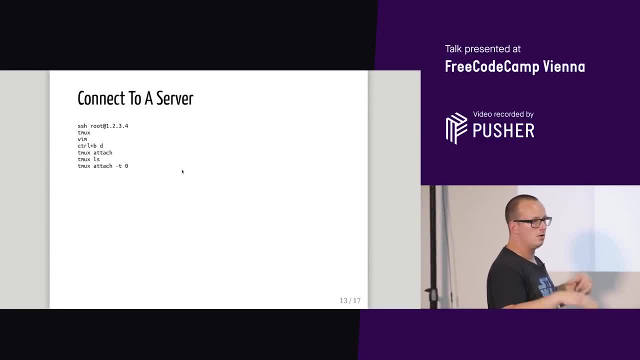 do some stuff in the server and then we close the connection. we go back again. the last session we had is gone tmux. a great tool like a new screen lets us open a session that we can close, and then we close this connection, we go back to the server. we can continue where we left off. you can also use tmux locally. 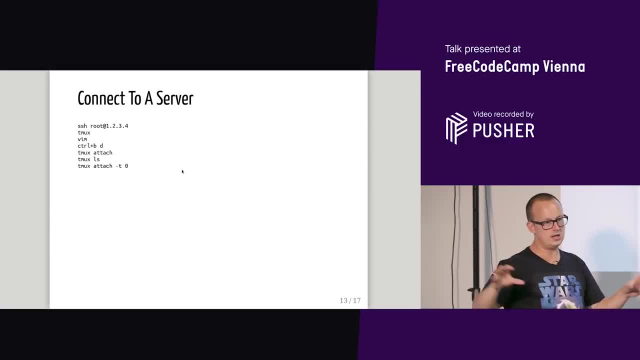 because it lets you split the screen in your terminal, different sessions, the sections, and it can be a good workflow, a tool. but it's nice to know that you can do that. and then vim again. you could, for example, have a workflow: you connect to a server, you do tmux to set up a session, you do vim to code some. 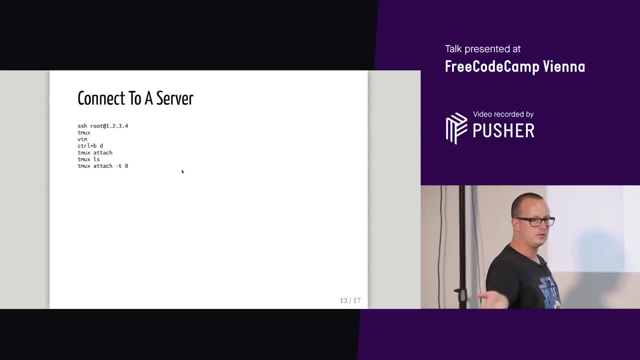 stuff. you leave it there, you go away. you can connect back in two days and hopefully the session is still there- unless someone's screwed with a server or it went down or whatever- and control BD just lets you, when you're in, tmux detach from that session. then you do tmux attach unless you have already more. 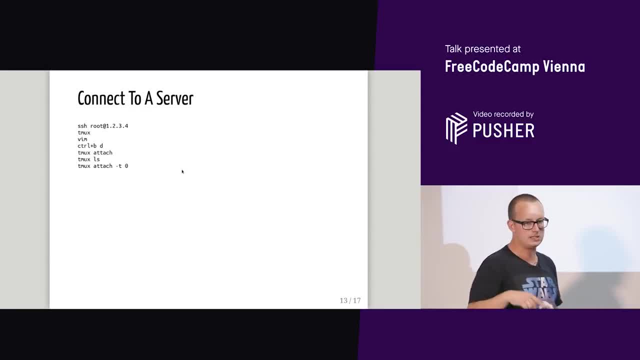 sessions and then you can do tmux LS, which is LS for lists, and you can see if you have more sessions and then you can selectively choose which tmux session to go back into. but this is more advanced, but now you know, but that's stuff, you. 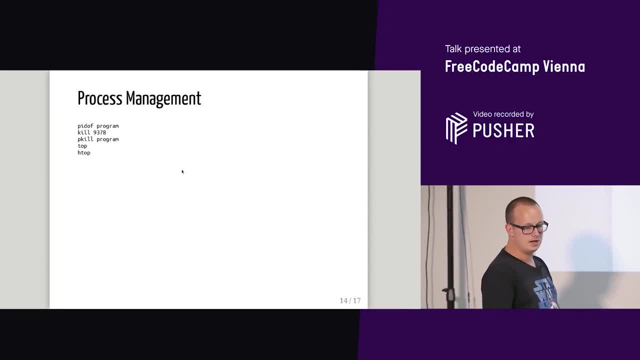 can do, I guess, process management, and now we're on 14 of 17 slides. it's not so much left awesome. there's a great tool that is not so often known about. I think that's called pidoff. so let me take a step back. in your Mac or your Linux, there's processes running. I don't know so much. 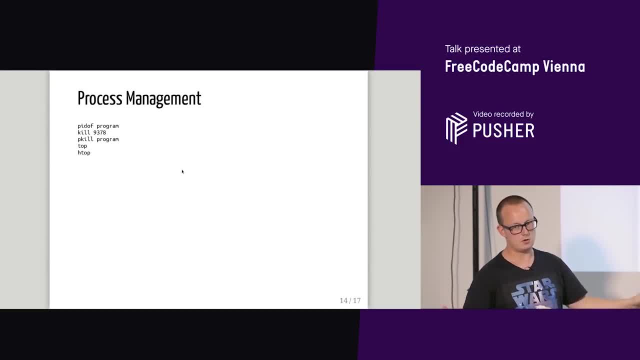 about the Windows world there. but there are processes, but they're managed differently as far as I know. so here you would want to, for example, close down your Firefox- that broke, or Google Chrome or your video player, like: oh stuff, froze, what happened? then you can go and have a look at for the, for you to instruct the. 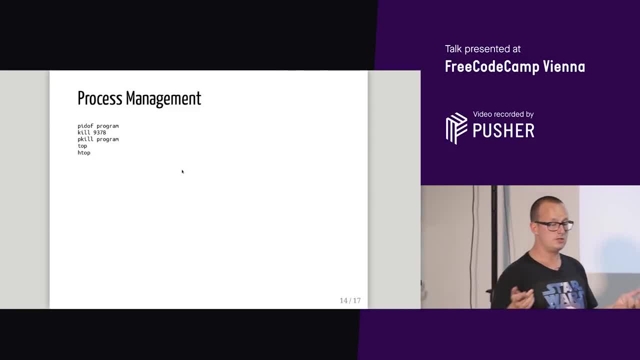 computer on what to do. you normally need the process ID. a PID is just the process ID of something, a program like Google Chrome or for example. you can just do PID of program instead of having to do PS, OAKS and more advanced tools to find and. 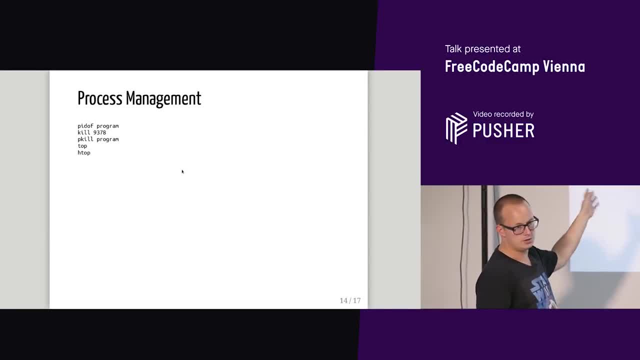 then grab for and stuff like. if you just want to do simple stuff, pidoff does a great job, it just finds you the PID of a program. then you get a PID like an ID, a number. then you can kill that number, that ID, that payment program, and then 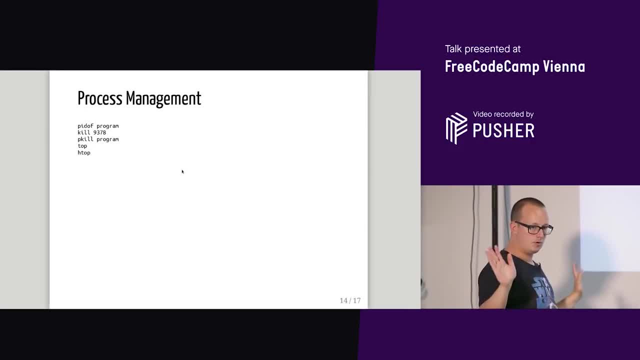 normally it just closes down and maybe your computer unfreezes. this is simplified because you would go more into depth in system administration. system administration stuff like keep track of stuff and have an idea of what have been sleeping and halting, and like what is hogging the most memory and the processors power, or 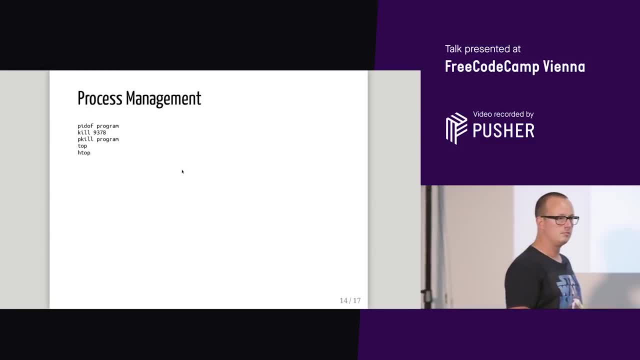 whatever it's called. top is a nice tool. that's always there. but if you do use Linux- or I think it's available with homebrew- you can use H top, which is a even more simple graphical user interface for managing this a little bit more with like f3 and f10 and searching and makes it easier for you, but it's. 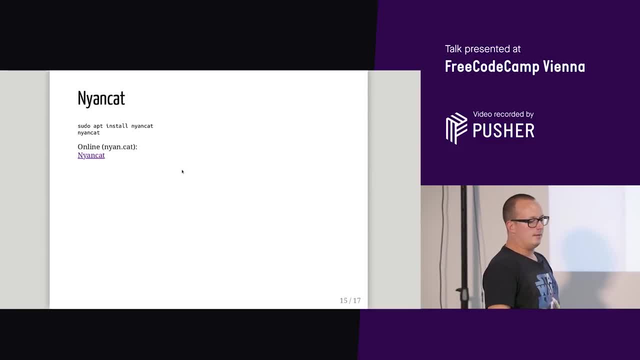 still in the command line maybe? yes, I'll show you this first after or actually the last thing we'll demo. remember? remind me to tell you about Nyan cat. it's a great surprise to finish the talk. you don't have to just be serious and all yeah. 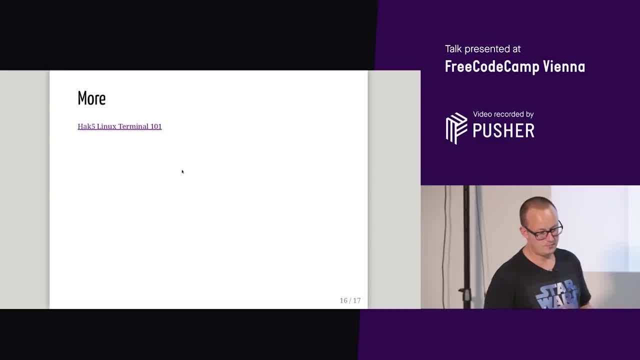 sysadmi with the command line. there are great resources and I mentioned these guys before. hack 5, H a, k 5. they've been around forever. they have tons of great videos, not just this playlist, but tons about if you want to get more familiar with the command line. 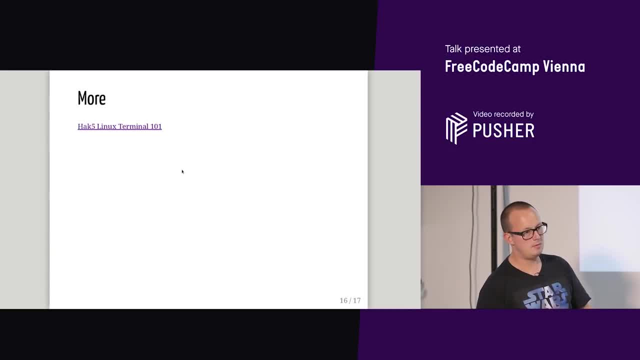 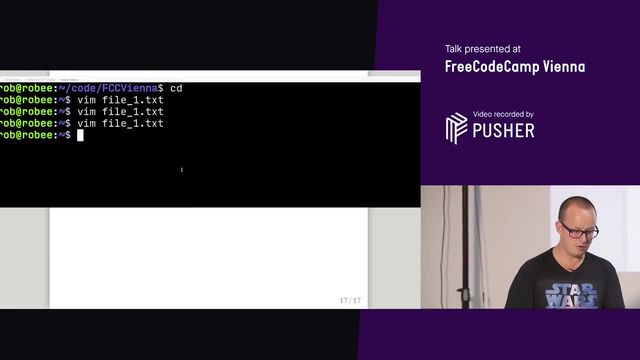 they're great at explaining stuff. they keep it simple, maybe just a couple of commands per video. it's really nice. this talk was made in Vim so you saw before the talk. maybe we had some like last minute like whoa, some stuff, I fucked up some, pardon my French. 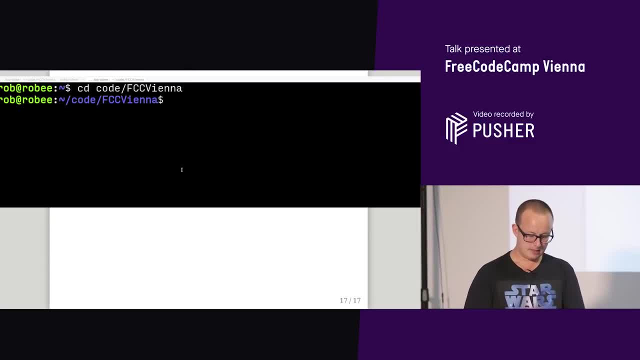 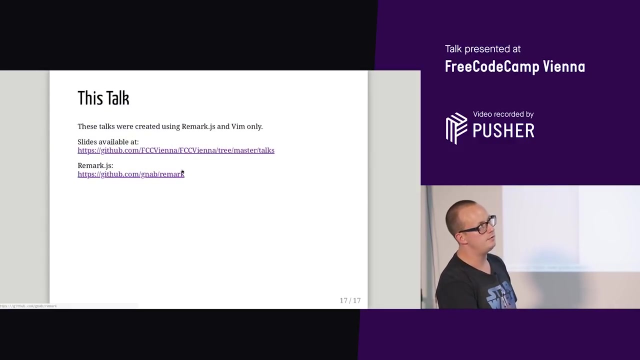 I. I managed to mess up with some stuff, so this talk is created in the command line the first time I do this, because I wanted something where I can just do that. it's an index HTML file that I'm just modifying in Vim and it's remarked as which is a library for doing slides in. 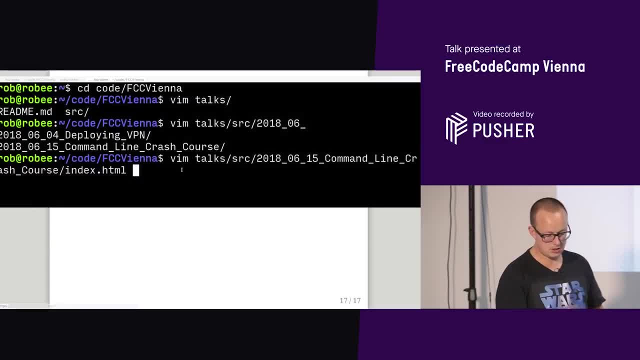 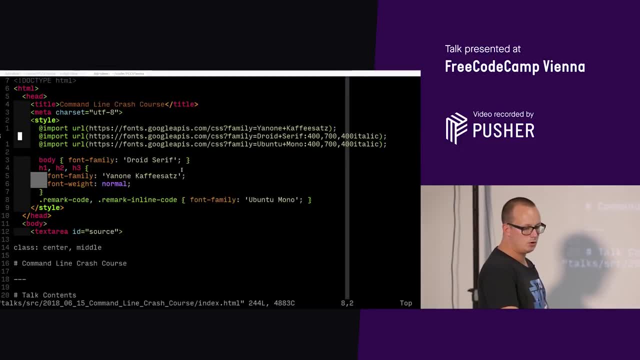 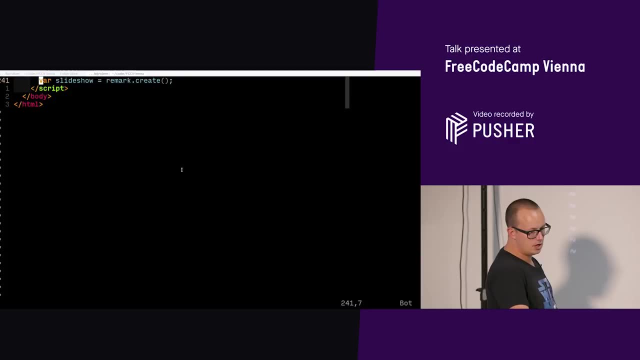 your browser and you just create, you just write markup. so you see is an HTML file with some stuff on top. it imports some font, then at the bottom it will then take the script needed for the JavaScript. so the slideshow script is this. remarked a s, but in between here all I'm writing is the. 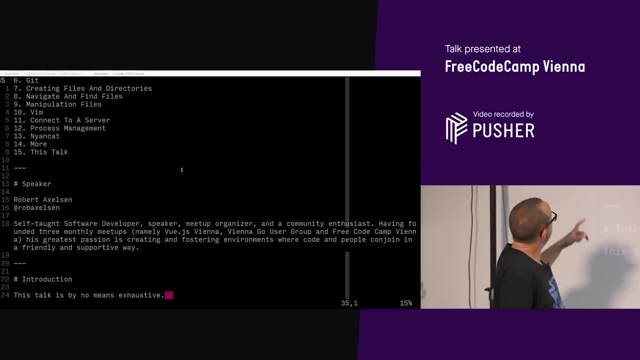 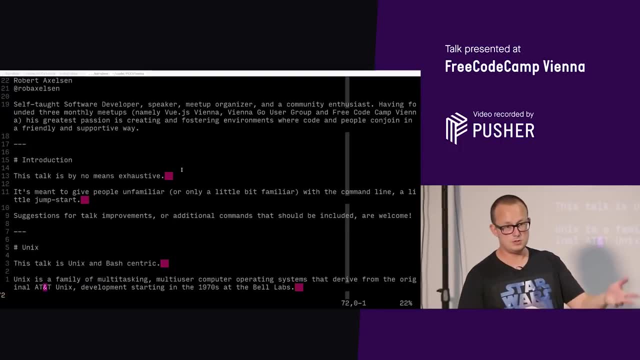 content of the stuff that you saw. now the whole talk is here, starting with the contents, and it's written in Markdown. My plan is to get a little bit more experience with this and maybe add my own style, but I really liked it this time around. 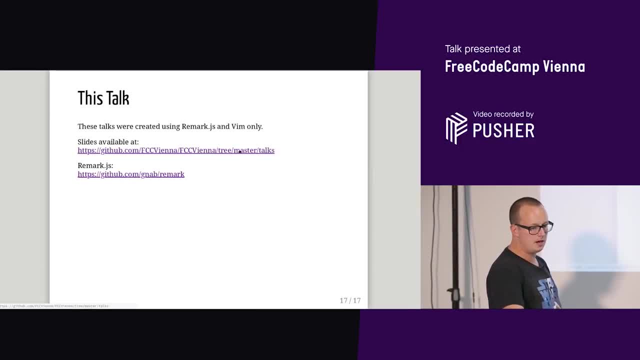 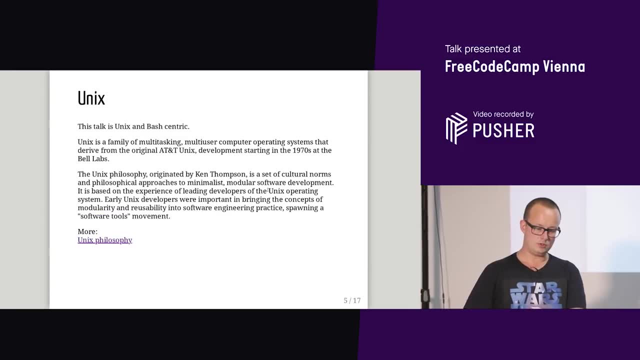 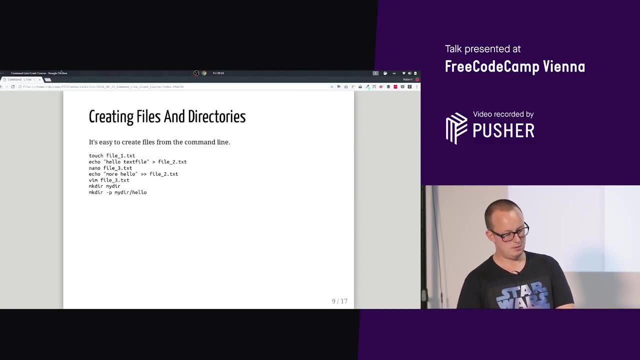 The slides are available in our repo for FCC Free Code Camp Vienna and Remarkjs you can check out. So I think we'll start by just having a short demonstration. We've gone a bit longer than I thought so we'll keep it short. 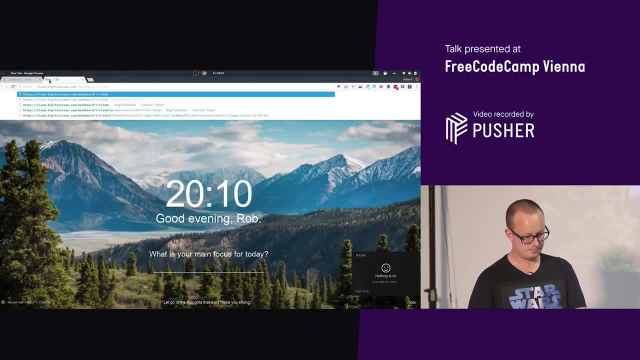 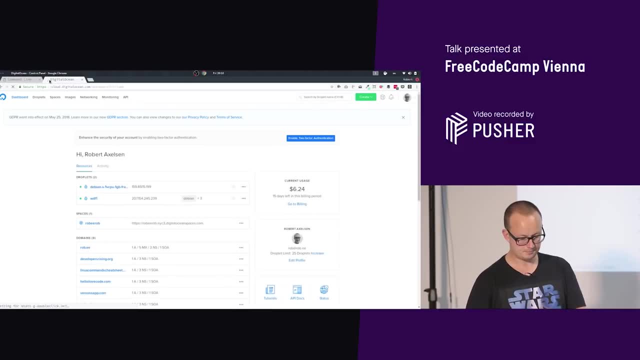 but we'll go to the server that I put up for us. We'll connect to the server and we can play around with some commands and then we'll try Nyan Cat in the end And after the talk, feel free to ask questions while I still have the stuff up. 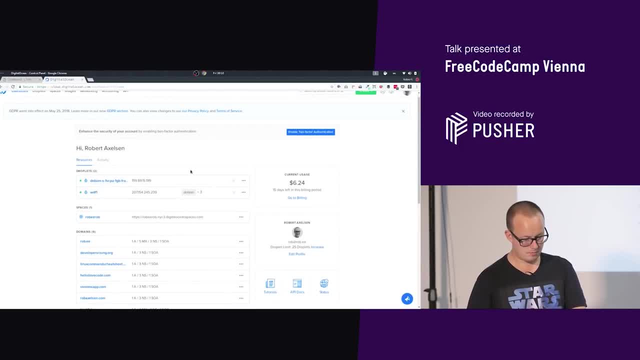 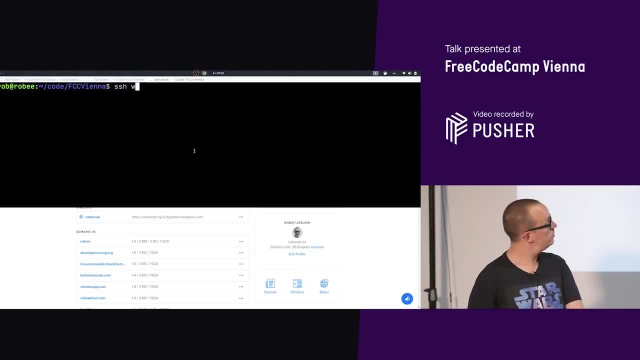 We can show something quickly if there's something related. So now I'm just don't let that confuse you, but let me SSH, like we had a command example, into a server. Is it big enough? Should I? is that a good? 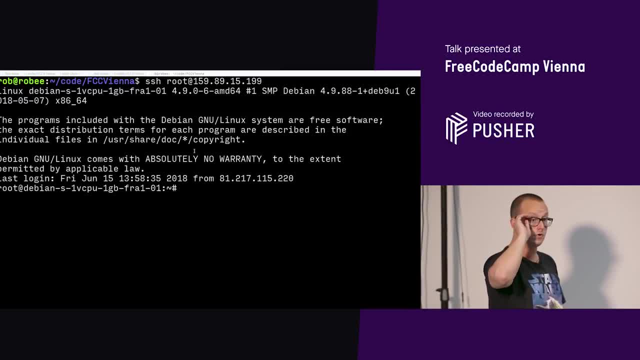 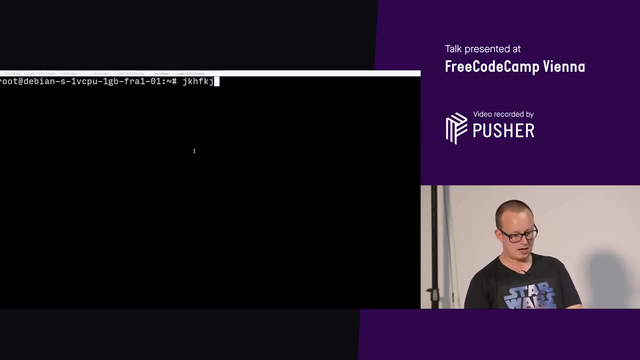 So now I'm connecting to a server in a data center in Frankfurt, So this is not my computer anymore. And here we saw the example of, for example, using Tmux. So I can use the clear command. I can use write stuff, control L. let's bash stuff. 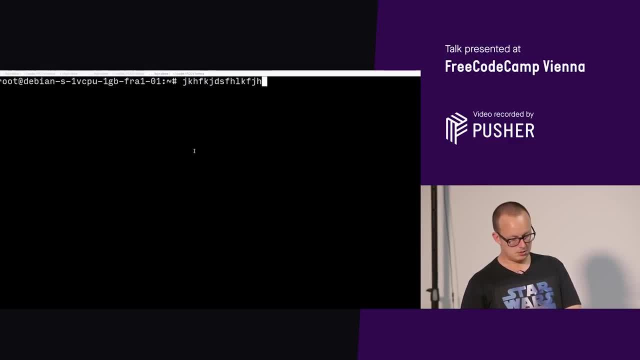 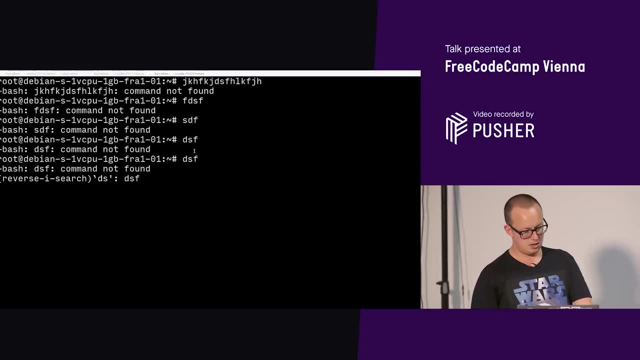 I can write stuff here And jump to the front, jump to the end. I can write some silly commands And then next time I drew control R. but this might not work this time around. Oh, it does. It shows us that the last time we started with D. 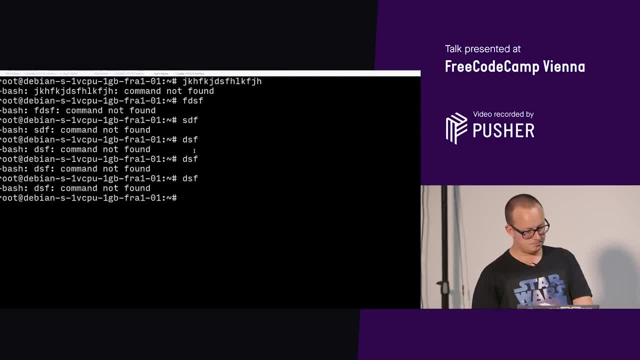 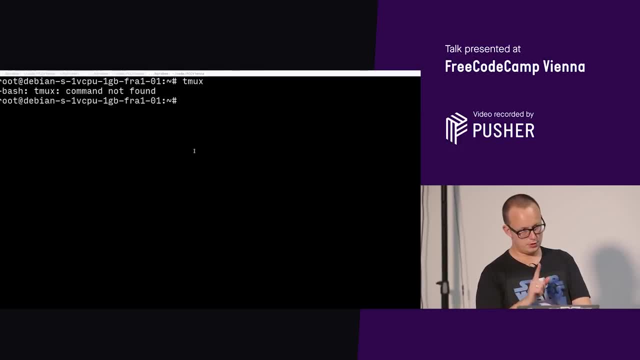 we wrote DSF, So I can do the same one again. Tmux, I won't show you that here then, because I remember now I was in the process of reinstalling it when my kid was hungry, So I didn't install it. 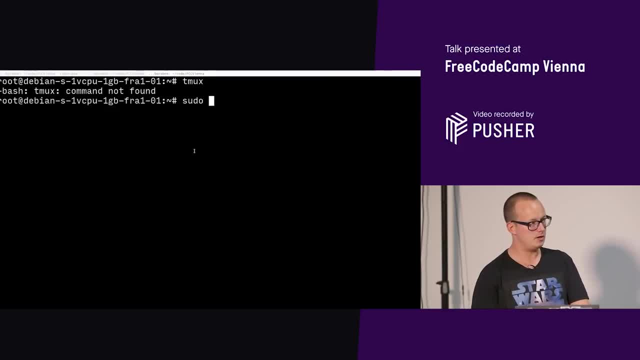 on the server. It will take a while because we have to update the whole cache here, but I'll show you Tmux afterwards And we could use Vim here to just. I think we'll take a step back and don't do that, because we will use it locally. 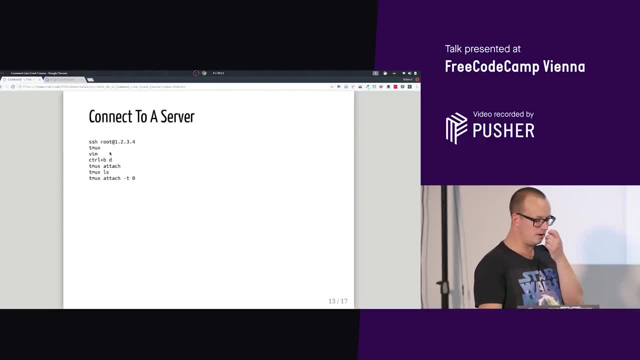 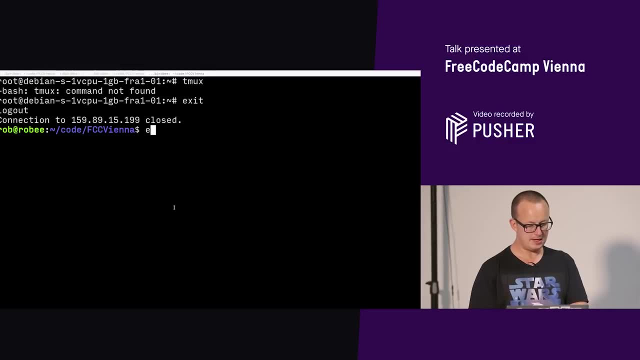 We did do the server stuff We connected to this server. I'll show you Tmux. Yeah, let's just go locally, for the sake of example. Let's pretend I'm on the server. now I can do Tmux. You see, there's even a command. 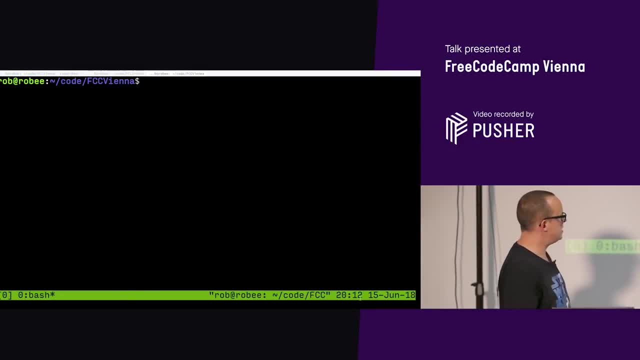 there's even like a graphical thing down here with some information. This might be some modifications here in my configs, But now I can do control like I can do some stuff here, right, I can do like I can even open a Vim session. 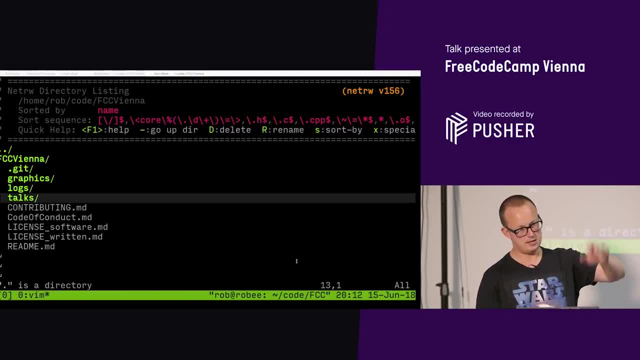 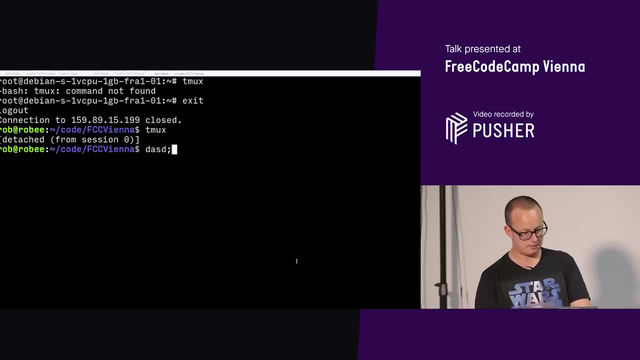 And then I can do. you see, there's stuff here, right? This is a list of the files there. Now I can control BD, I'm out again And I can do stuff. you know, I can even close this window and stuff. 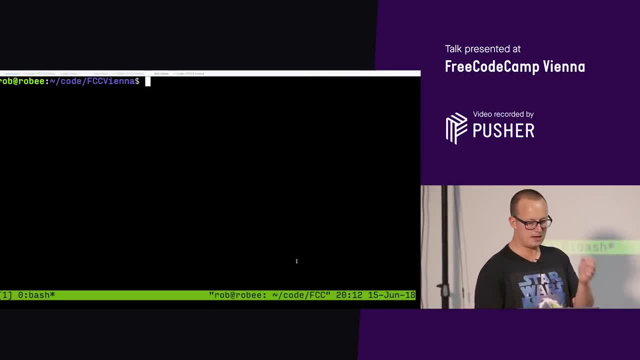 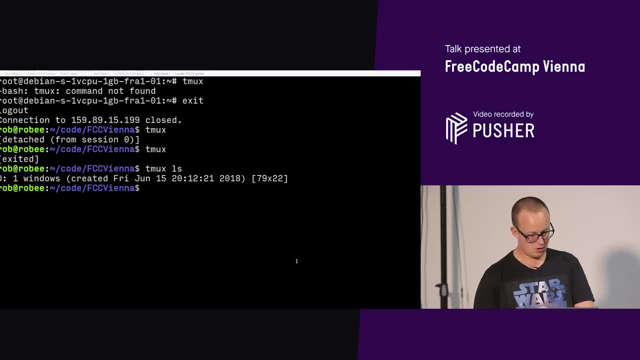 And then I go back. If I don't do anything else, it goes back to the. it doesn't go back to the same place, So Tmux. So it tells me there's a window open and then I can now go. Tmux- attach. 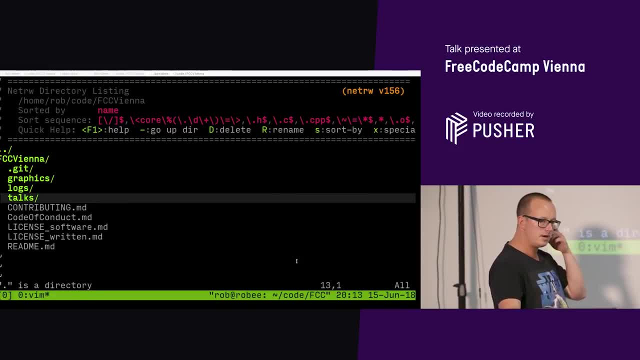 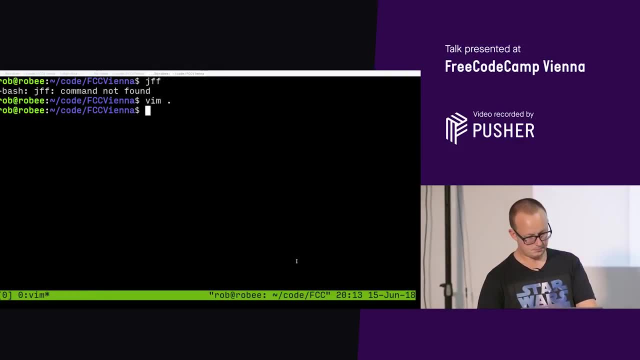 T0, and now we're back to where we were. So this stuff is still running in the background. Normally, if you close the terminal, it's gone. in the Unix world We can see, for example, pidoff, and we shouldn't do it on Google Chrome. 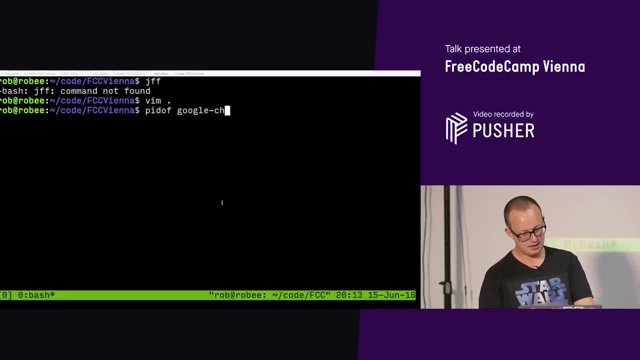 because it has. it's a bad example. It has a lot of Chromes here, a lot of tabs and stuff. I think it's maybe stable. Let's do Google Doesn't work. Let's do pidoff tilde. Okay, this terminal that you're seeing now is called tilde. 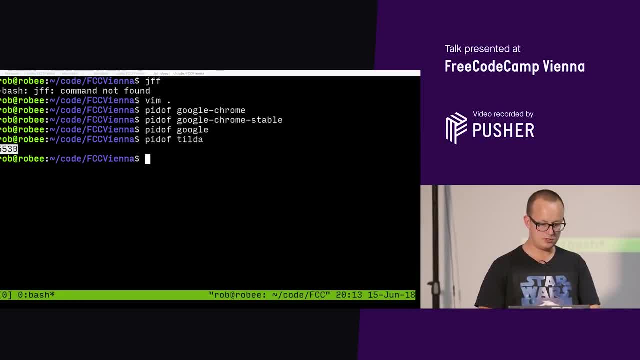 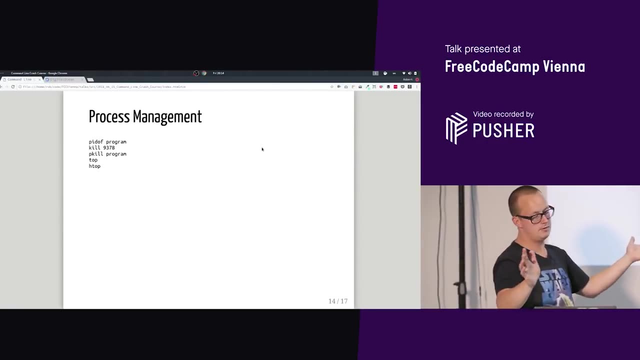 I knew it was there. It gives us this one. Let me just check. if there's some stuff I don't want to close here, It's fine. So if I now do kill this one, the terminal's gone. Whoa, It actually did what we told it to do. 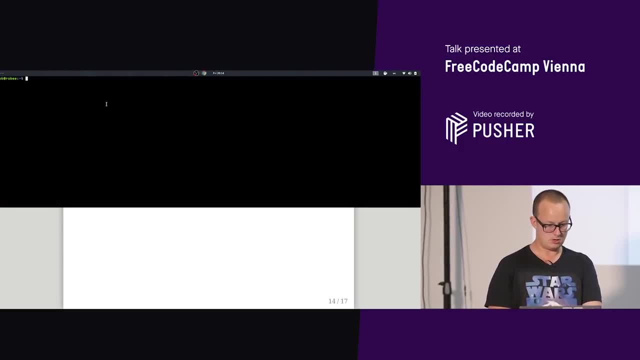 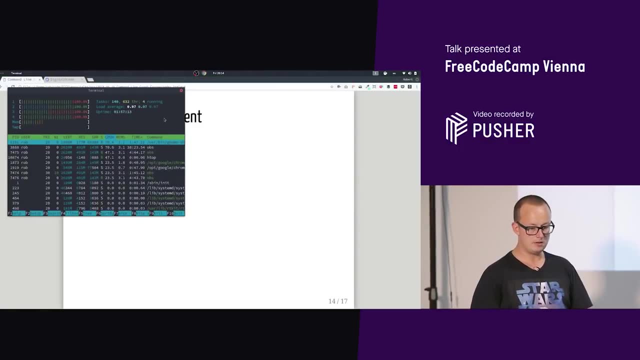 And because I killed it, I have to take it up again. So, okay, that was one example, Just to show you a different one that you can. this is still the command line. This does the job of telling us all the programs that are running here. 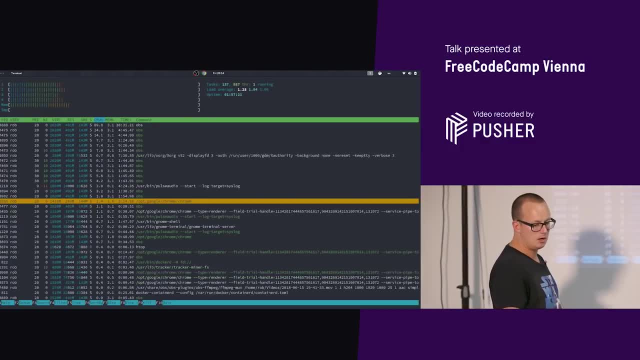 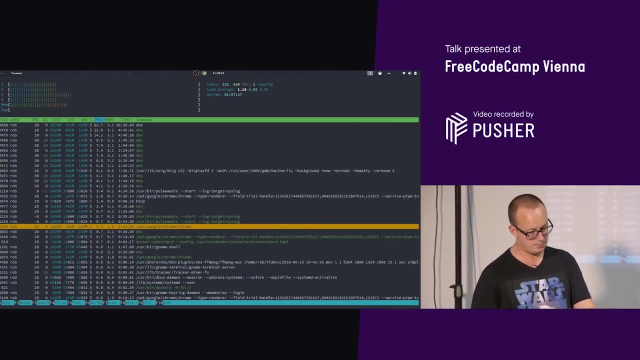 I can even search for Google. Give it a name. It gives us the one on top here And I can kill Google Chrome now And this is easier because you see the shortcuts down there And this is easier to navigate around, especially if you're new to the command line. 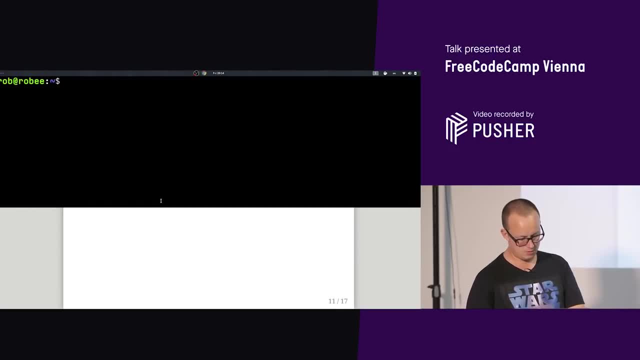 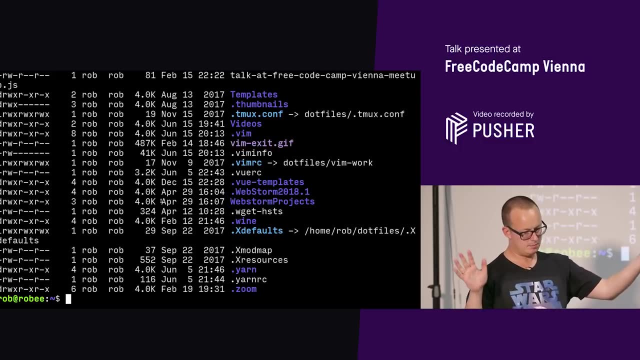 I think we'll just create a file and then we'll do the NAND cat and we'll finish. So I am here now. I'm listing out all the files here. I'm listing it in a better format, using flags so we can see the size. 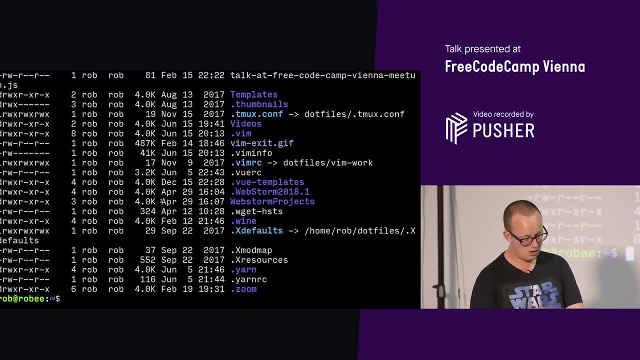 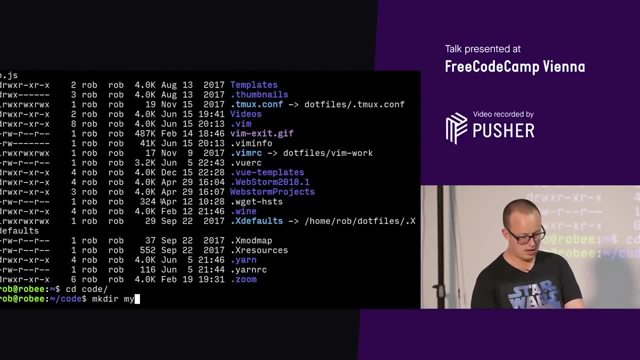 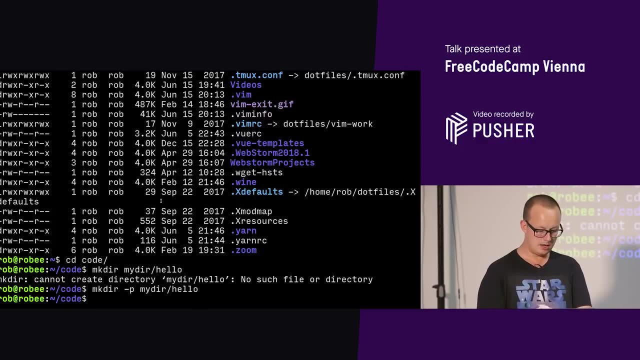 I'm listing it in a human readable way and so forth. Then I want to go and make a directory. I do my dear hello, But it tells me you can't create it because my dear doesn't exist. So we use the flag we talked about earlier. 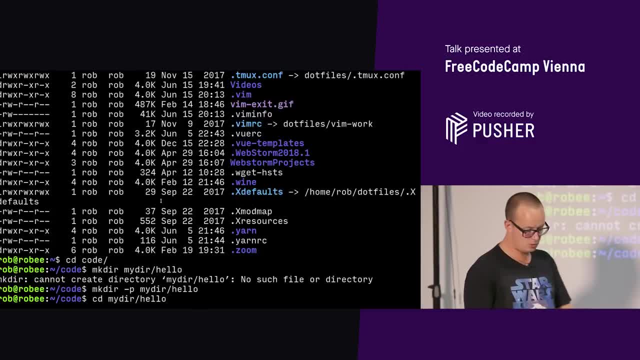 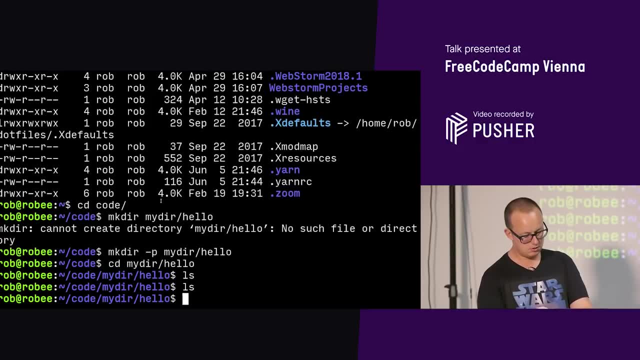 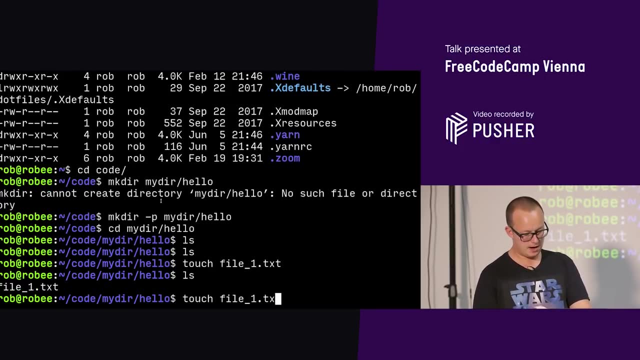 Now there exists, my dear hello. Is this too small maybe? Now we're here, Now I can touch a file. So there's nothing here now I can touch a file. Now there is a file living here. I can touch file two and three and four. 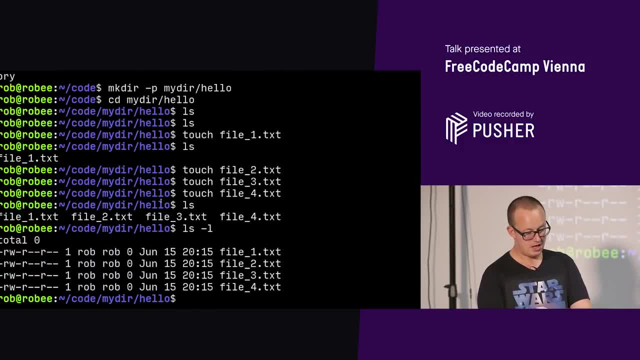 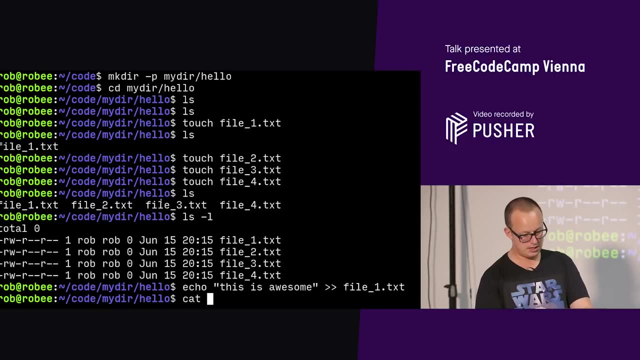 Now there are more files here. I can list them like this And then I can do echo. This is awesome And I can put that into file one. There's another command. It lets us just print out everything in the file to the screen. 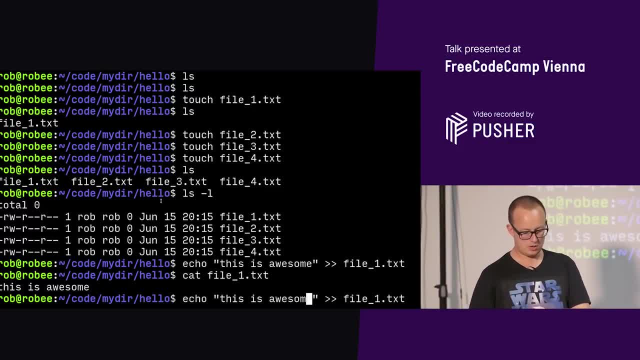 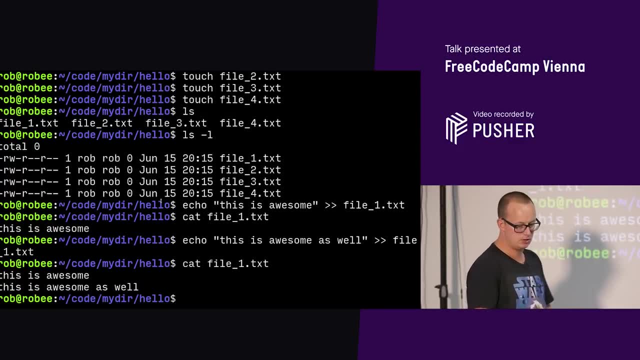 So we see, this has now. this is awesome. Then I want to have another file, another line in that file, And it shows us: this file contains these two things And we can figure that out again with vim. So it shows us: now we can edit this stuff. 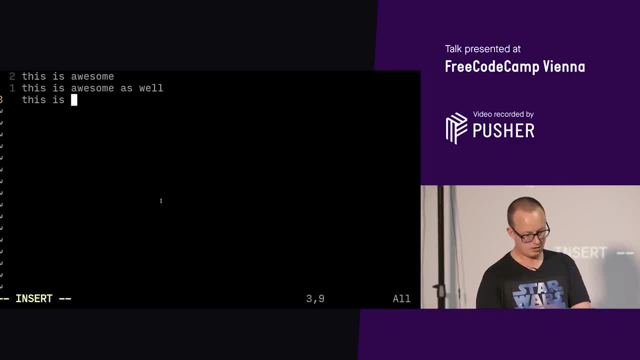 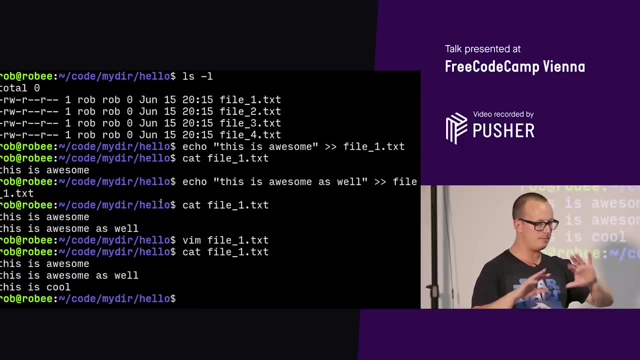 and I can add a third line. Awesome, it's there. So I'm using the command line, just using the stuff that you saw earlier. It might seem like magic when I'm doing it, And I'm even using control A to go back here.